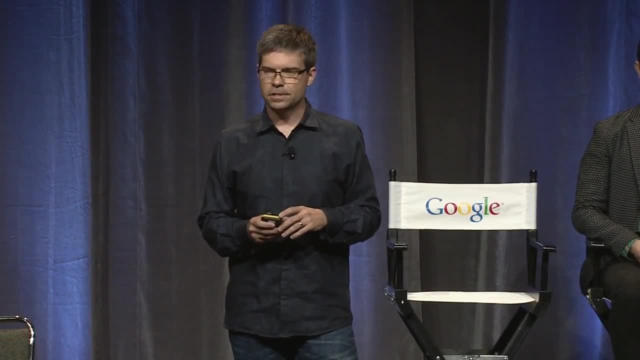 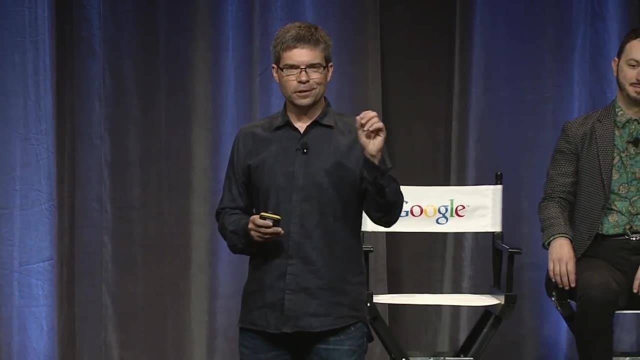 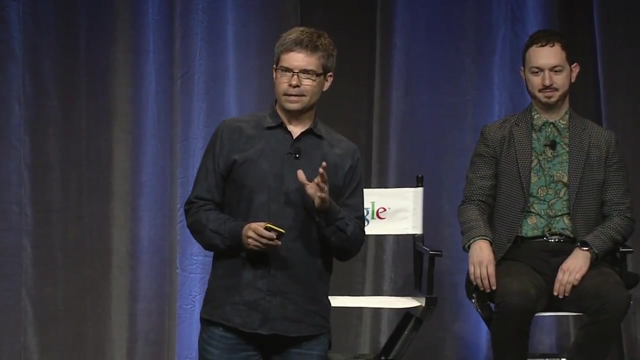 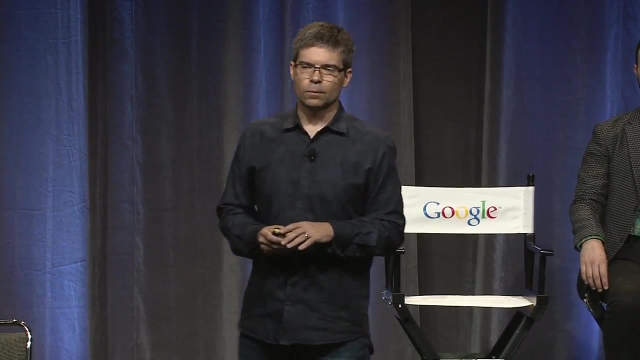 classic concepts of good design, with a solid understanding of the most fundamental physical properties. At first we thought like designers- How should it appear, How should it look? But then we thought like scientists: Why does it behave this way? And after many experiments and many observations, we wrote down everything that we'd learned. 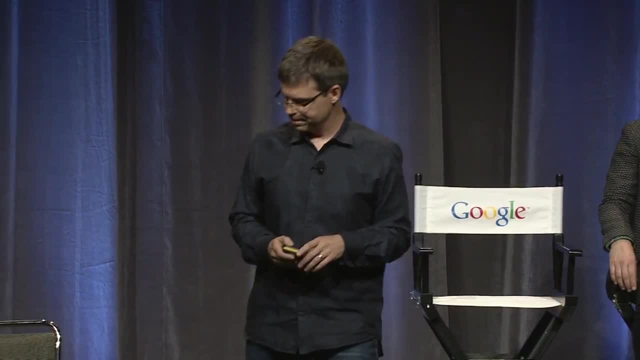 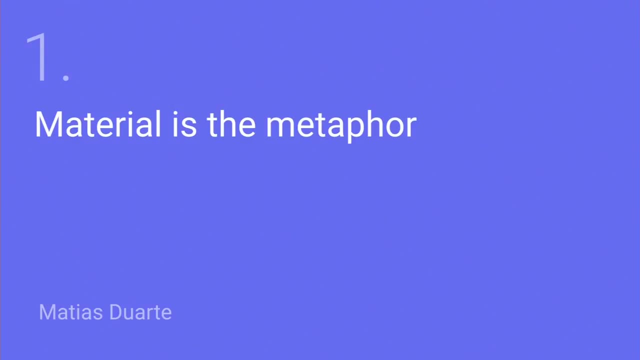 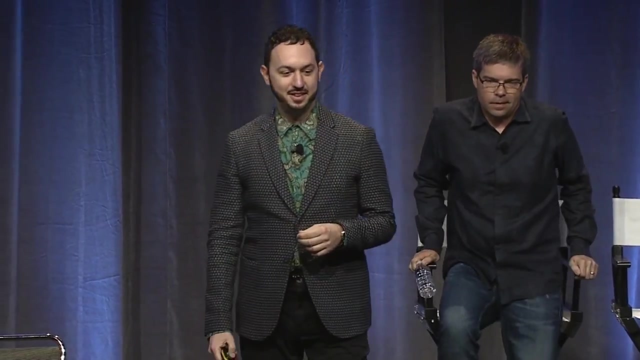 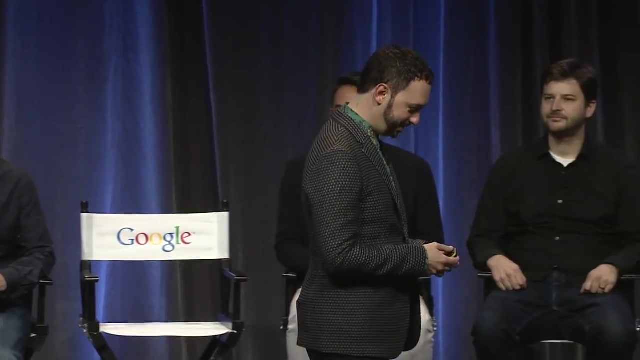 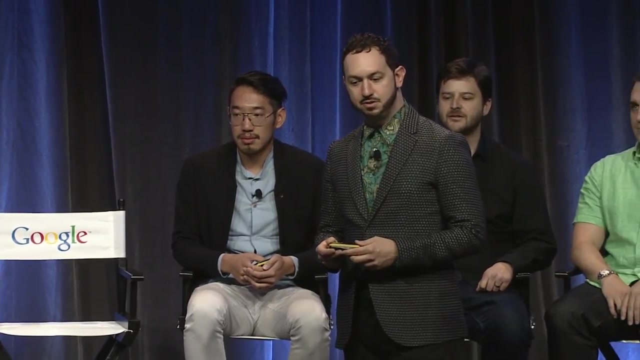 These are our material principles. Thanks, John. Yeah, Hello. In Android 4.0 Ice Cream Sandwich, we introduced a typographic, magazine-style UI And a lot of people liked it. We were pretty happy with it, But design is continually evolving. Users are getting more sophisticated. The design 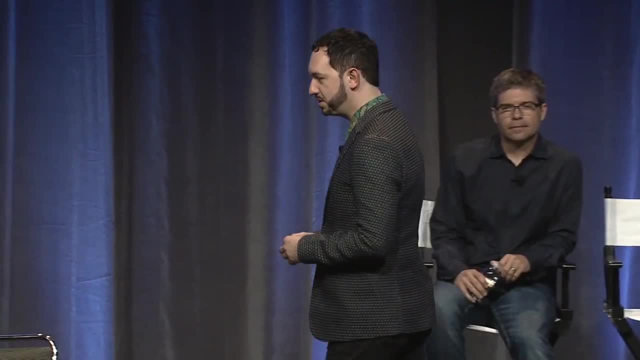 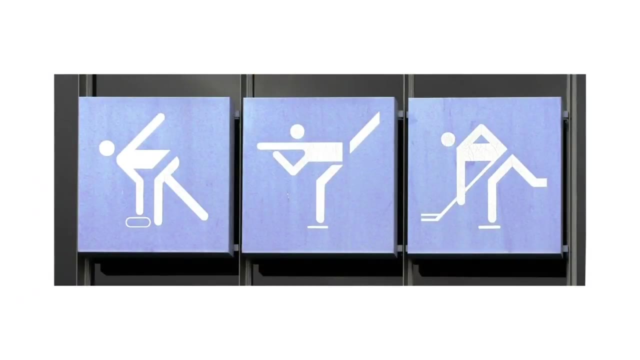 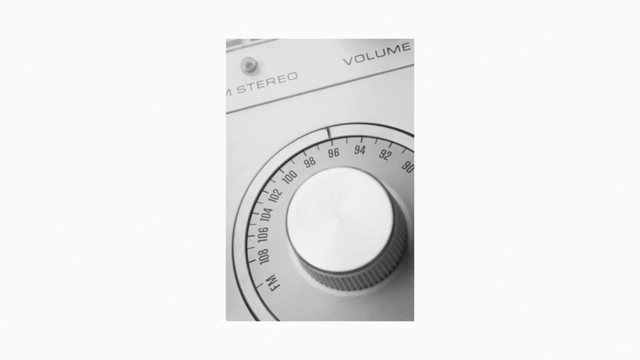 landscape is more sophisticated. In particular, motion has become incredibly important over the last few years. We wanted something that was taking the very best out of the design, of graphic design, clarity and the innovations in motion graphics and motion communication, but that still tapped into those elements of tangibility, of physicality, that industrial 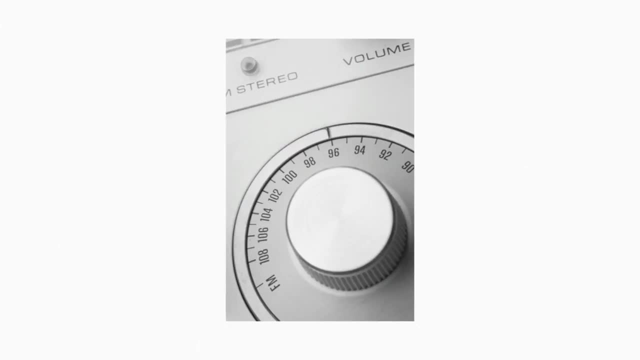 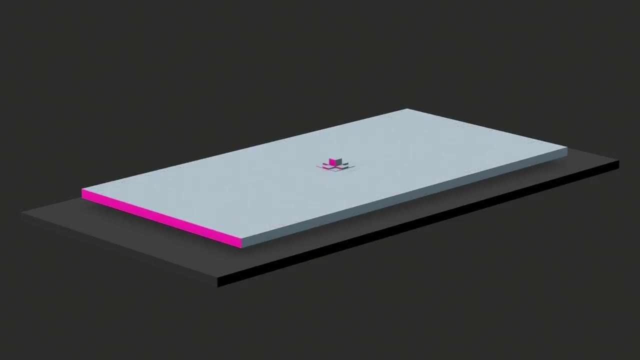 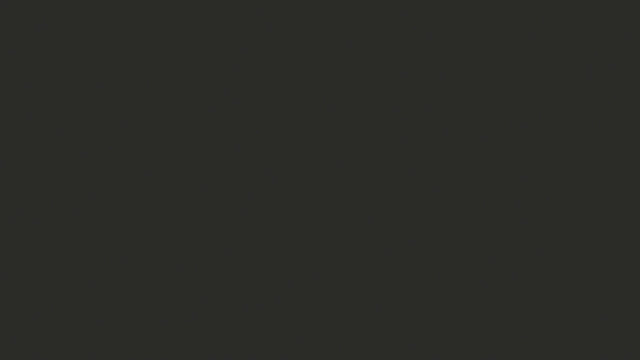 designers themselves use. So this led us to a question of how do we do this? Yeah, Yeah, So the very first principle in material design is metaphor, which seems a little random. Why metaphor? Metaphor is basically a very, very short story. 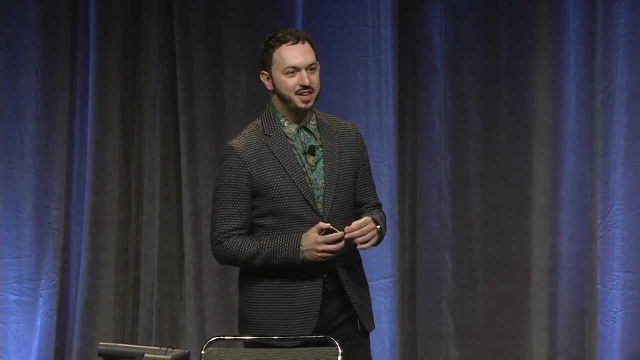 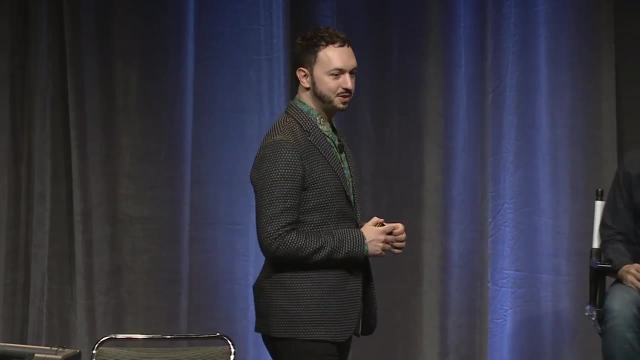 And, like stories, metaphors are really powerful because they are deep and dense in meaning. They communicate more richly than verbal language can. When I say: if I'm writing a play, if I'm telling you about a character or a person, 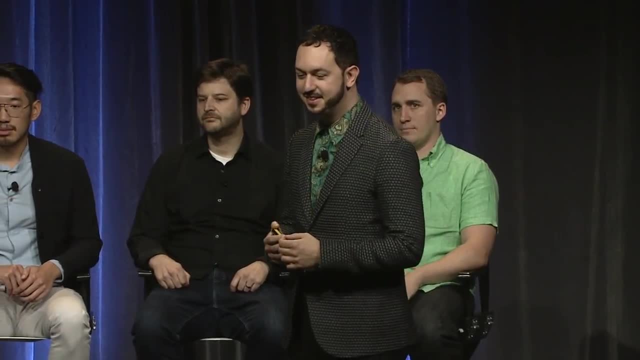 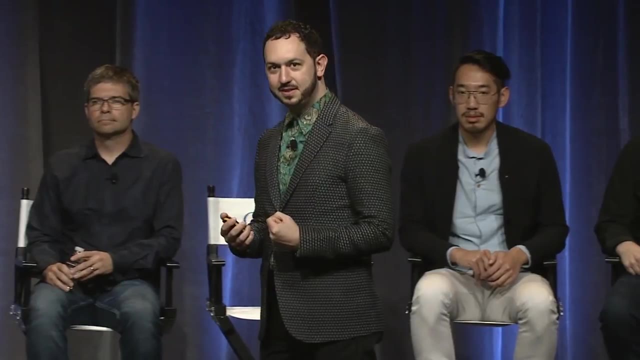 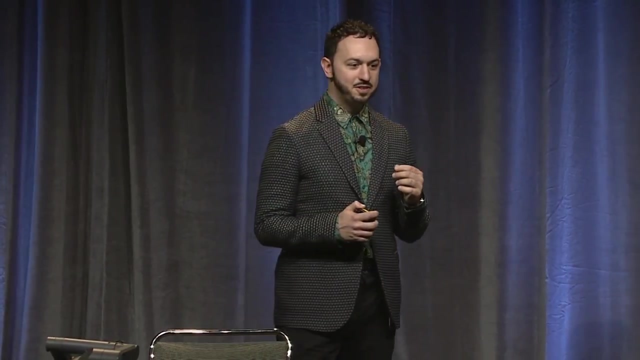 in real life. if I say she was a hurricane, I don't have to tell you about her force of will or her indomitable spirit. I don't have to tell an actor that averting her gaze would be inappropriate. The metaphor is a form of knowledge transfer that depends on shared experience And in 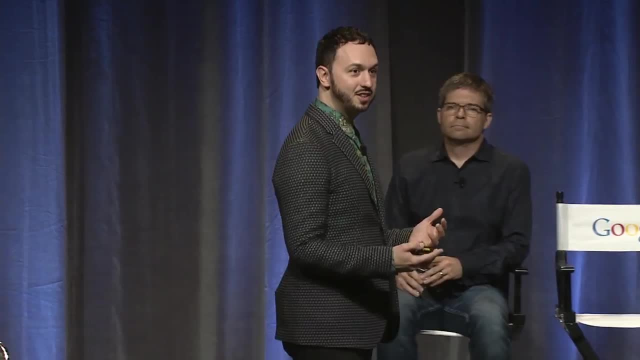 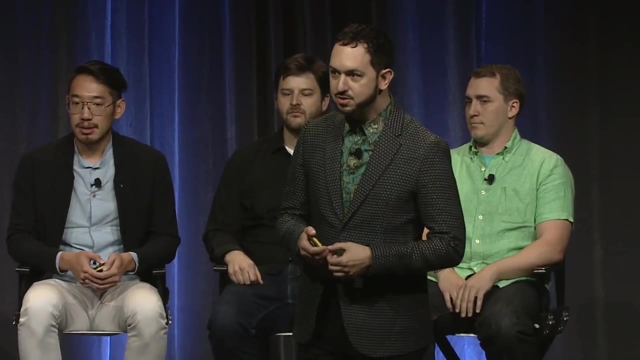 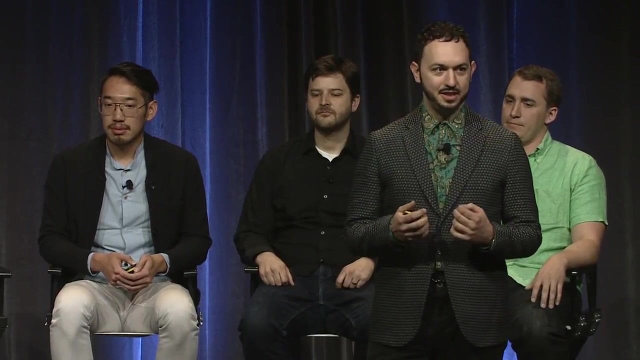 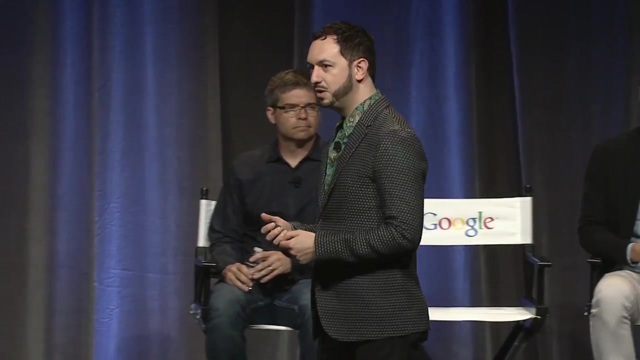 fact, this capacity to transfer knowledge and to transfer learning is one of the things that defines humanity And, in fact, defines intelligence. So for us, the idea of metaphor is a back story for the design. It unifies and grounds the design, And it has two functions: It works for our audience. We want to present a metaphor. 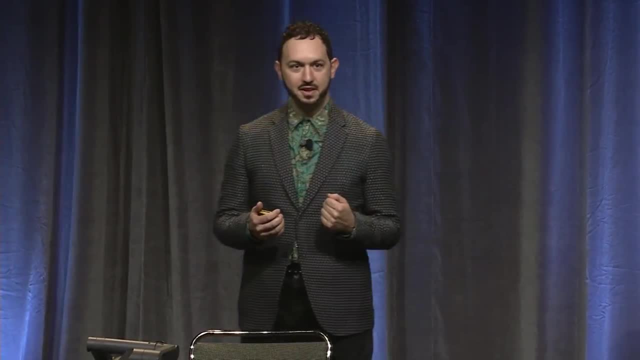 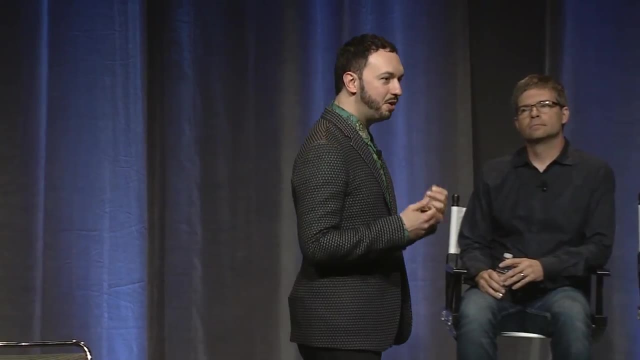 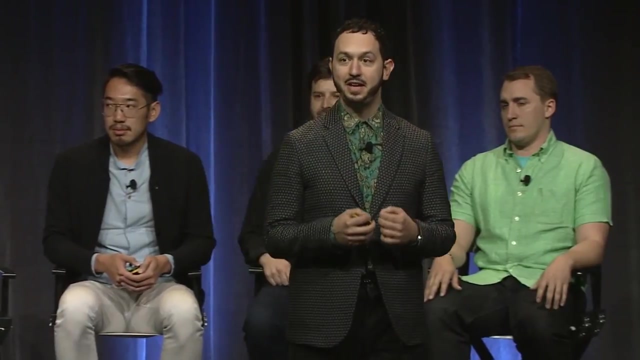 that they can understand, that they can connect with, that they can use to move faster into understanding how to use things. But it's also a metaphor for ourselves, for the designers and the developers and the PMs and the QA people, everybody working together. Because when you have a metaphor, 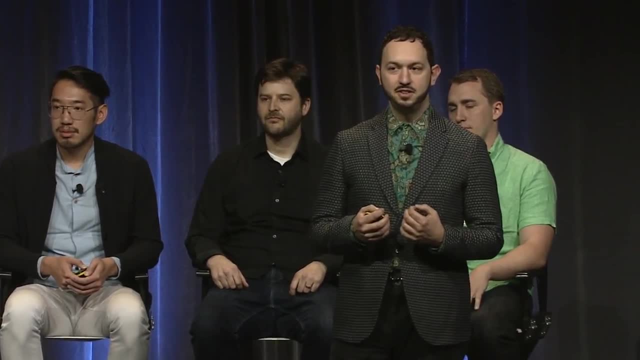 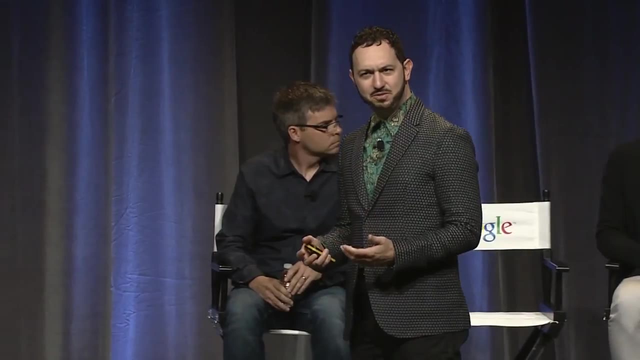 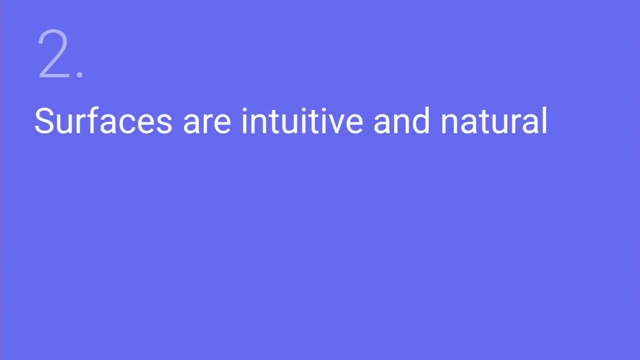 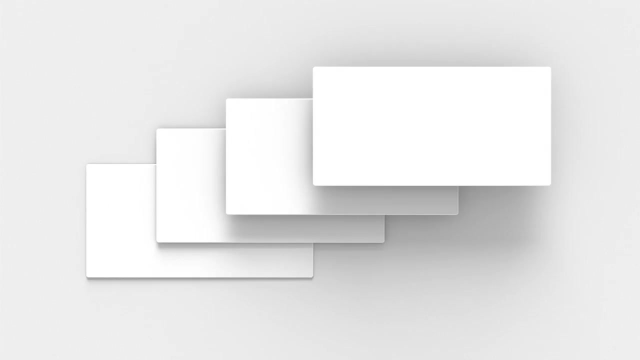 that everybody understands, intuitively understands. you don't have to explain how they violated subsection C, clause 2 of your style guideline. They just know it feels wrong, They know it's out of place. So why this particular metaphor? Why did we imagine a material that was a form of paper sufficiently advanced as to be indistinguishable? 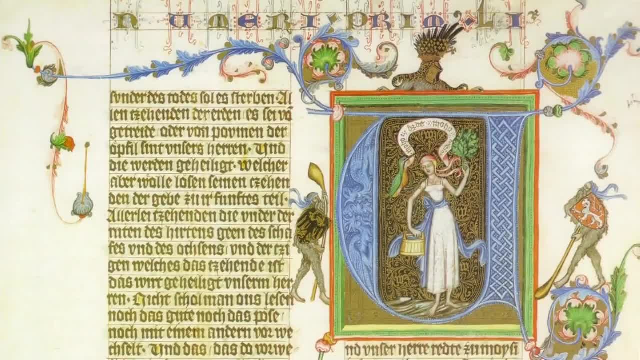 from magic. Well, one part of it is, of course, that we do have a lot of experience, as humanity, communicating with paper. Paper is just rich in a history across all our cultures of conveying information, and it naturally affords so many different ways of interacting with it. 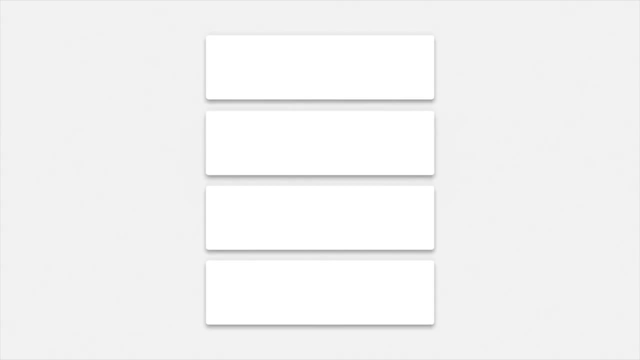 But the other aspect of paper is that it is a physical thing, It exists in the world, And this idea that surfaces, because they're tangible, are a metaphor that we can use to accelerate understanding of our UI is really important. You have this perception of objects and surfaces that's happening in the more primitive parts. 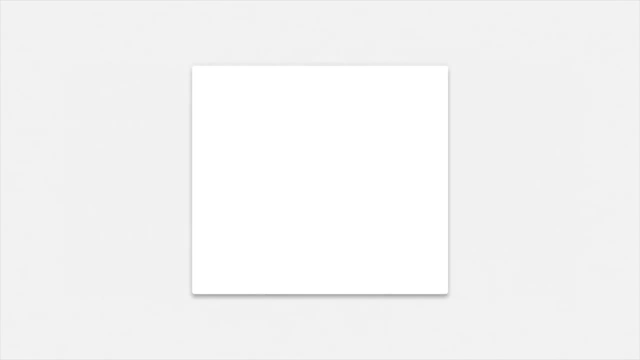 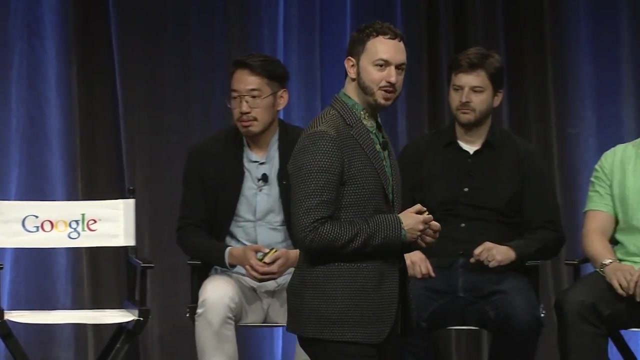 of your brain. It's happening in these visual cortexes that are in the back and lower parts of your brain, And that means they're tangible. They're simply easier than language. They are more natural than language. You have this inherent understanding about the separation of things and the relationships. 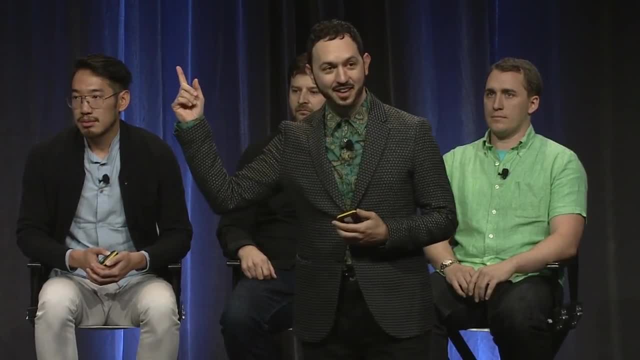 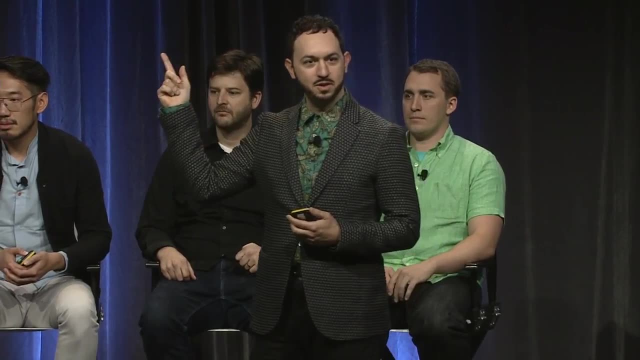 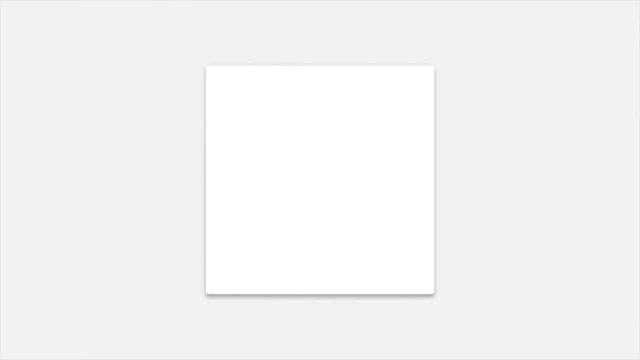 of things that allow us to look at this and have it make sense, Even though we know there is no material in the world that could possibly do this. It is irrational and yet feels completely natural, And that's what we want when we're creating our own. 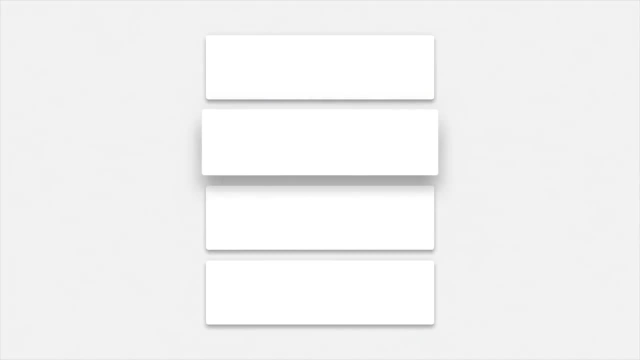 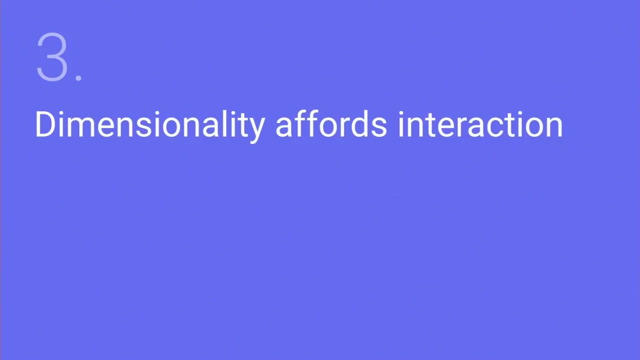 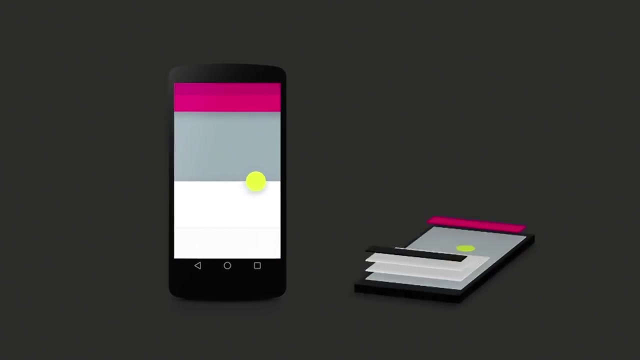 Thank you. digital, magical interfaces: right Because we are not constrained by the laws of the real world. in our user interfaces, Surfaces are intuitive and that's why we use them as the foundation. They organize space and rationalize the interaction. 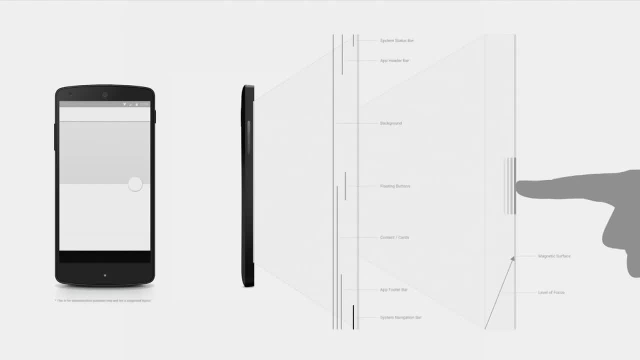 And it matters that you preserve this inherent sense of what's right, not for the sake of artifice, but in order to make the mind work less. One of the things you'll discover in our material design documents is that our buttons rise to the surface. 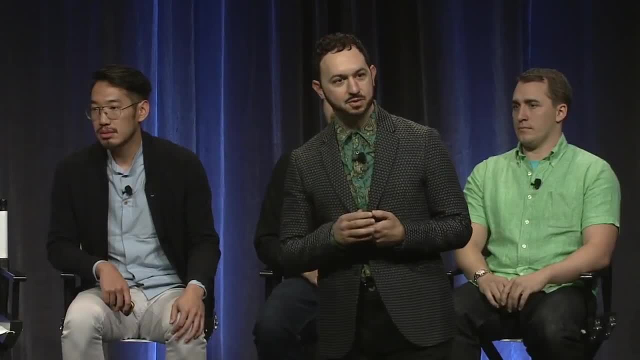 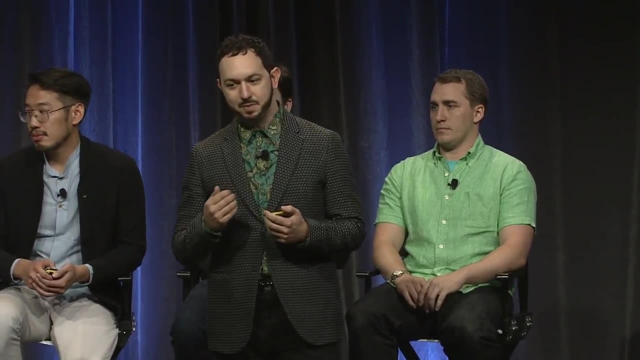 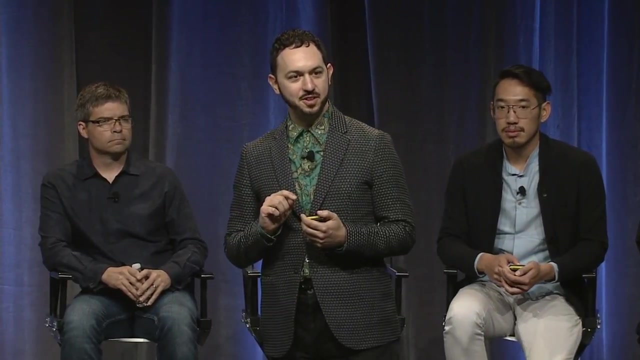 in response to touch, Instead of sinking into a surface like a fake plastic button would. And we do this because we want this illusion to be consistent: The idea that when your finger touches that glass on your phone, that surface is coming up and meeting your finger. 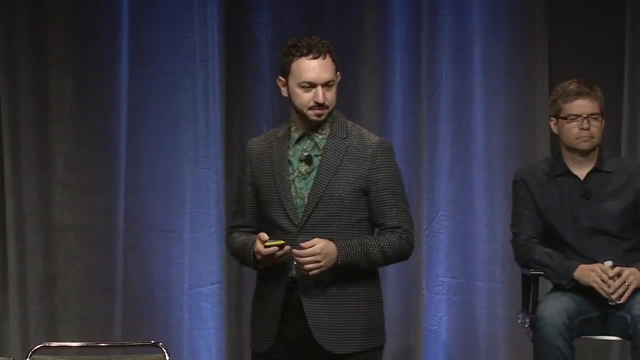 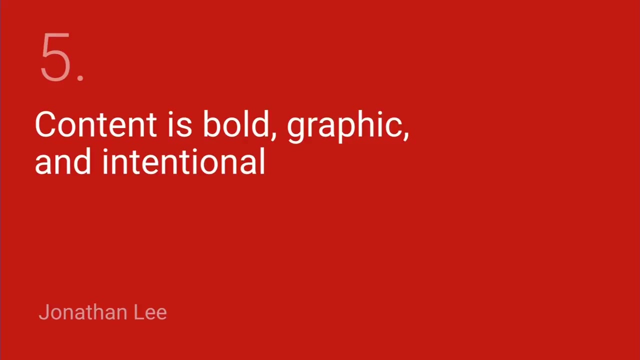 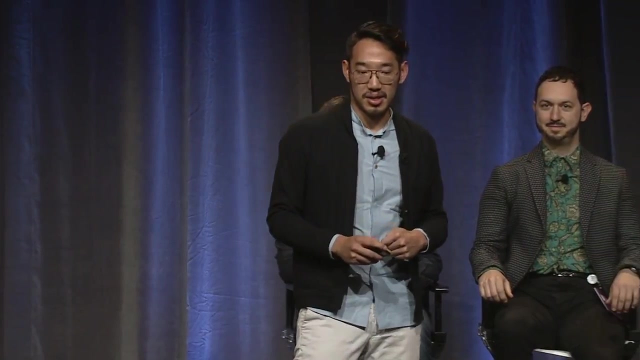 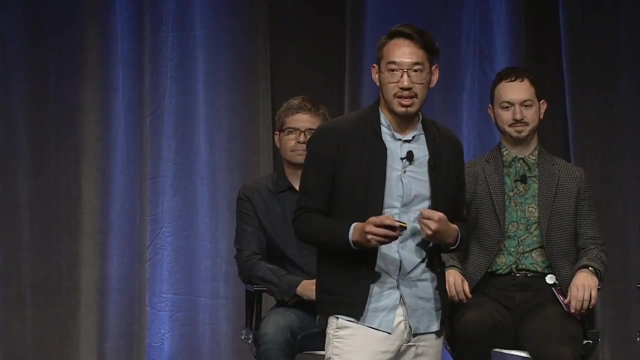 at the point where it touches. Yes, All right, thanks, Matthias. Question: Content is bold, graphic and intentional. We pushed ourselves, when we were thinking about material design, to make clear and deliberate design decisions regarding color and typography, So embracing these classic visual design principles. 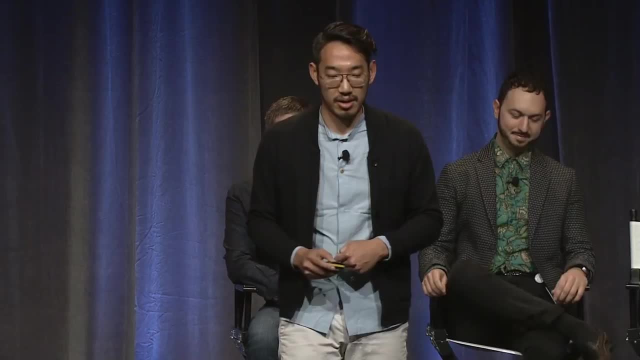 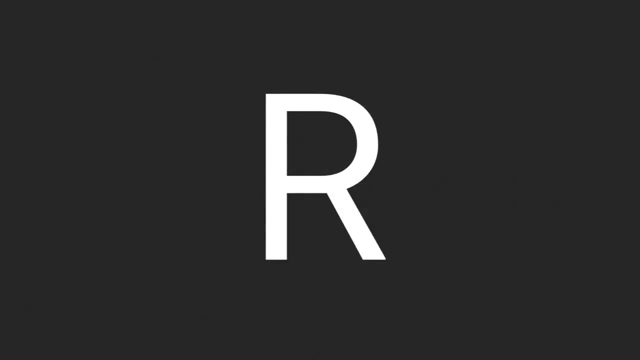 that John and Matthias have both spoken about. in our new framework With Ice Cream Sandwich, Android introduced a new system font, Roboto, And today we're updating Roboto to go beyond phones and tablets and be the default typeface for the material UI. 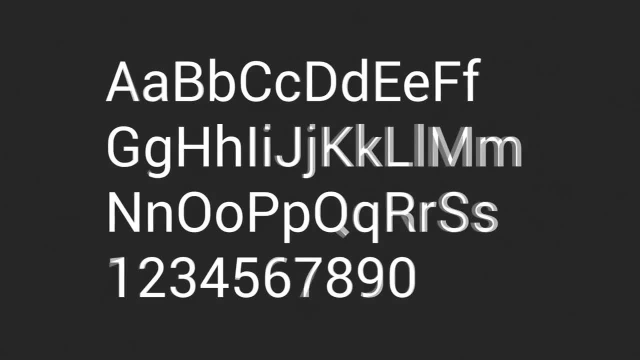 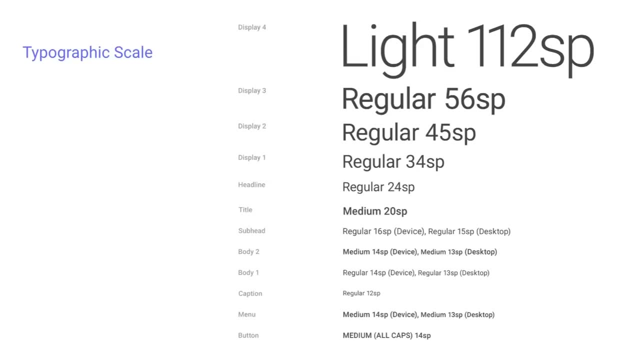 Here you can see the current version of Roboto, And Roboto is now slightly rounder, friendlier and, most importantly, redrawn to perform on desktop and beyond, And I can tell you from personal experience that it handles really well. We also developed and documented our design guidelines. 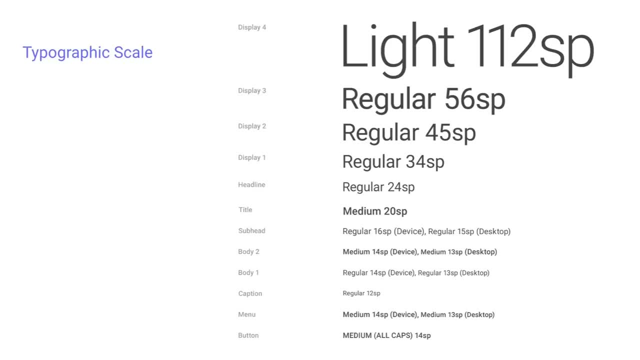 for typographic scale By using one typeface and a handful of weights for emphasis. we believe that it's going to be able to do a lot more. It delivers consistent and clear hierarchies in your products, Using scale and appropriate display sizes. 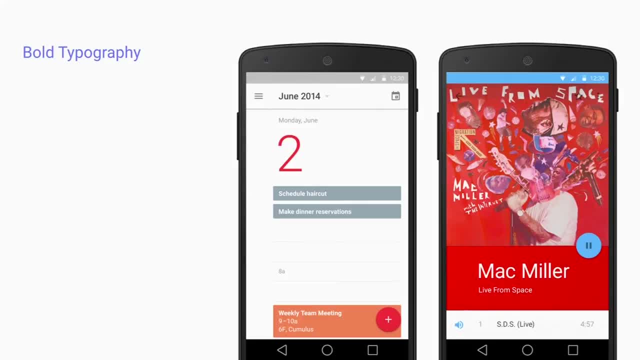 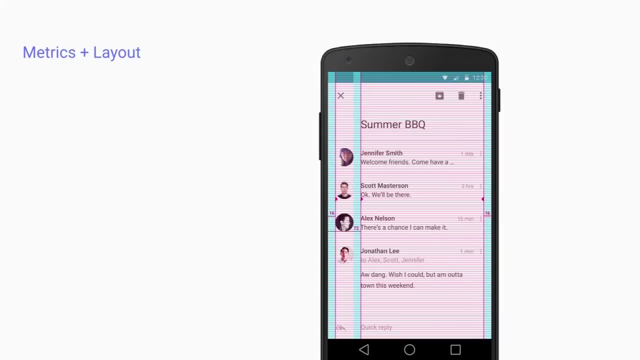 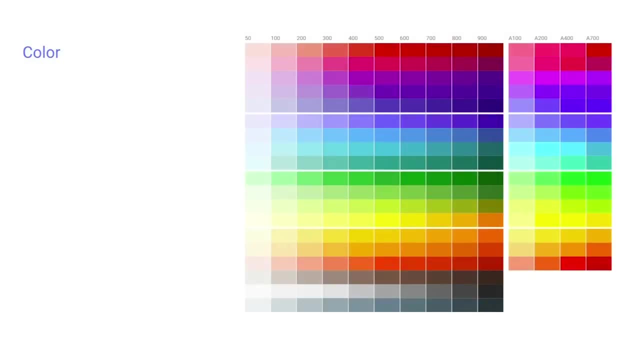 you can create dynamic print-like layouts with using white space and contrast. This focuses your users on the content that really matters. Using vertical key lines and baseline grids, content is bold, elegant and graphically clear. We also developed a complete color palette with intentional 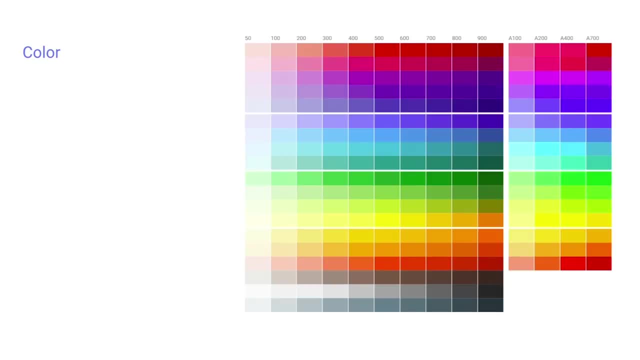 color decisions for shades, tints and accent pops. These are not just adding white and black to a color or using alpha. We actually looked at each of these shades and decided what they should be. So strong and intelligent application of color gives life to your UIs and it connects users with your brand. 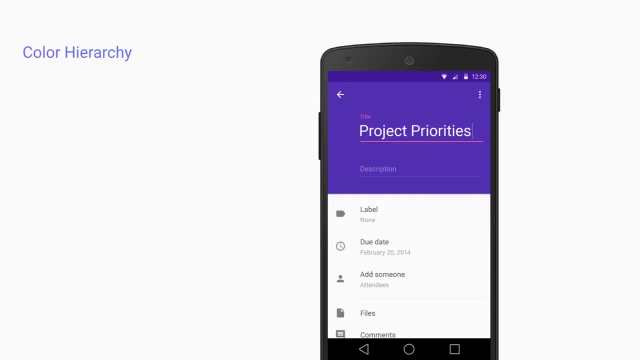 It also can create very strong hierarchy and liven up some pretty standard UIs. As you can see in this example, it's essentially some kind of form that you're filling out and there's a a clear area for your title and that's. 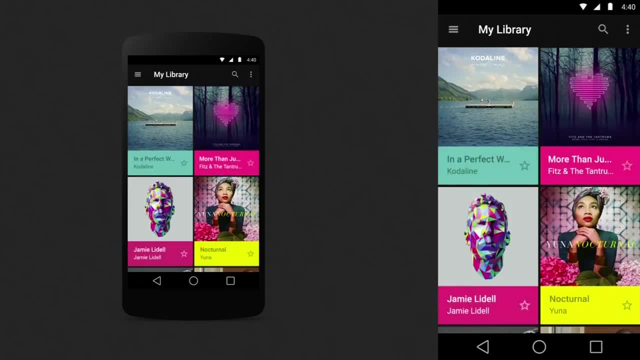 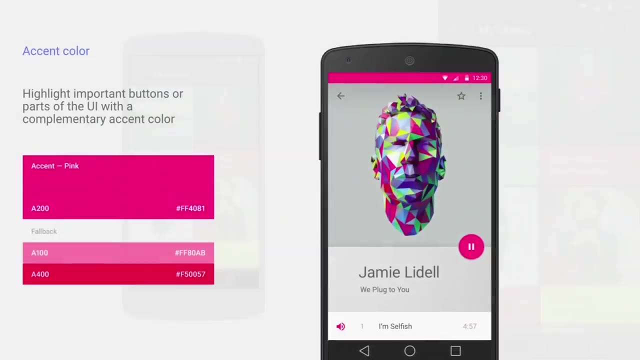 what we want people to focus on. Dynamic color is also really exciting. Earlier today, Matthias announced a new API in the L preview called Palette. This system really makes it easy to color things dynamically, select and extract color for use- One of the things that you could use color for. 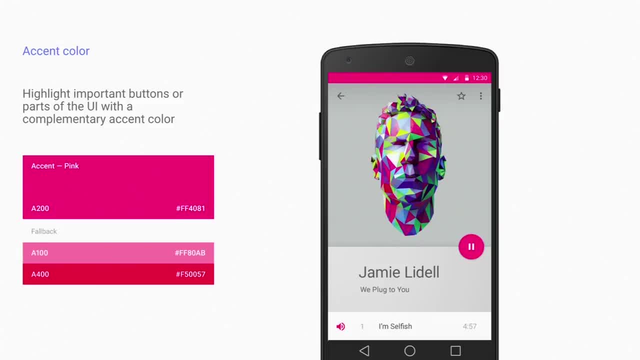 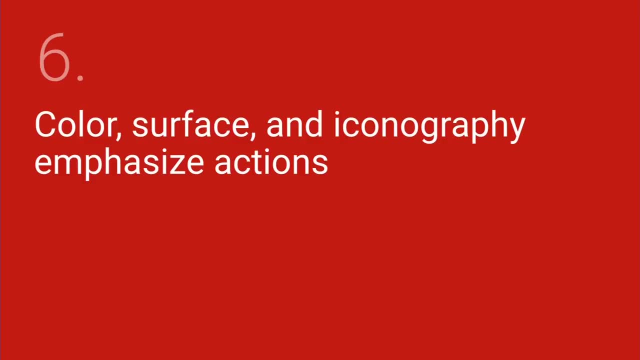 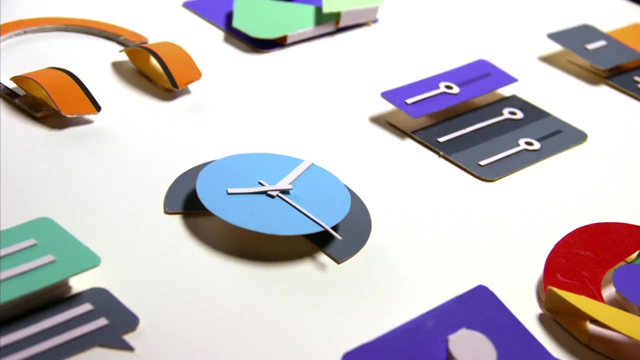 is contrast accent colors, Contrast colors. make this floating action button, which is the play pause button, really pop. Brand color and icons are accelerators that guide users through your design. When thinking about app icons, we looked at real life studies. 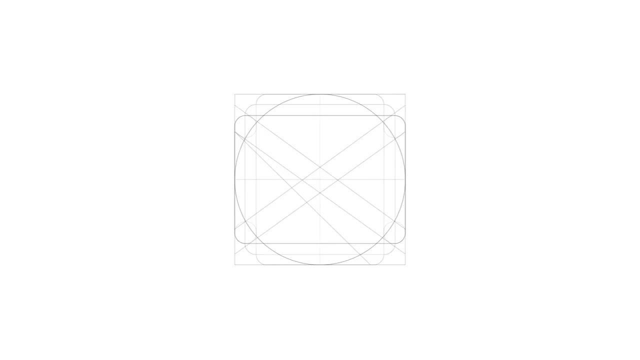 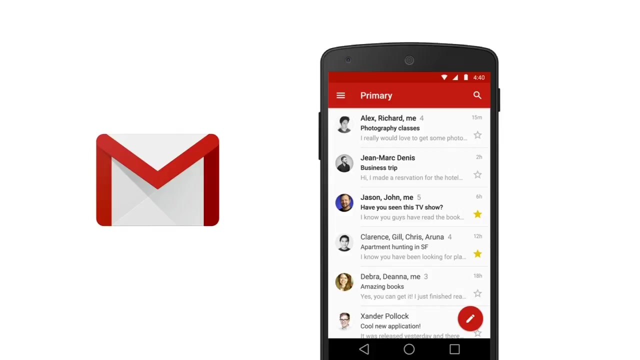 in lighting and shadow. We started by defining a universal grid for app icons, one that supports primary geometric shapes. A product icon is the first, least literal touch point of your user's experience. We looked at extracting those attributes from your icon and from your brand and intelligently applying those. 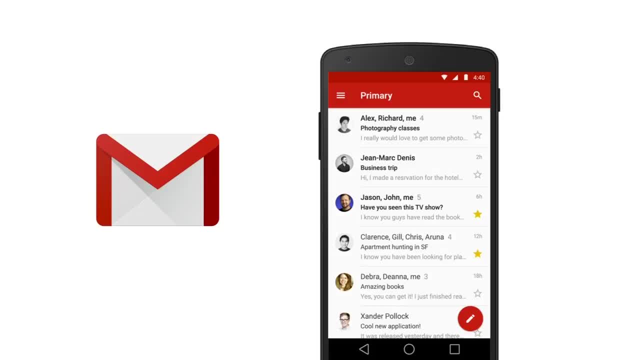 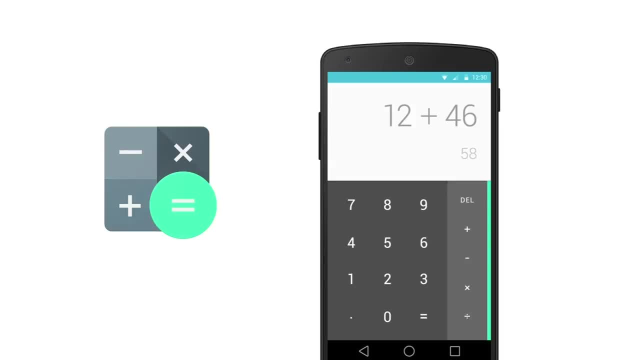 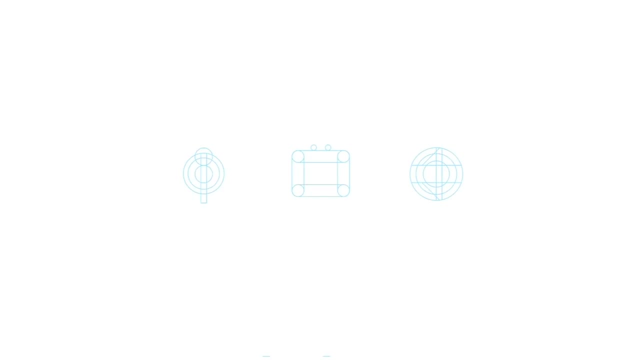 to the surfaces within your UI. The top toolbar and the floating action button again are accelerators for those actions. Here's just another example of how to connect those surfaces to the product icon. And finally, we took the same modern, bold, geometric. 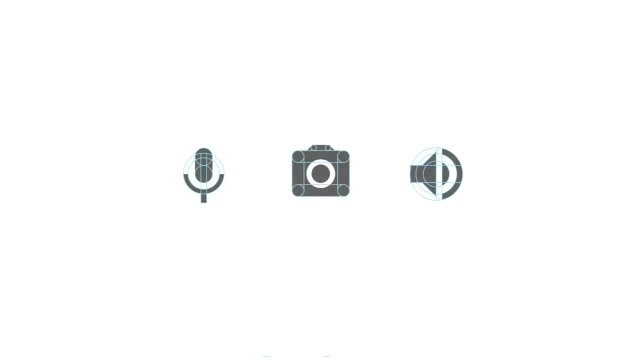 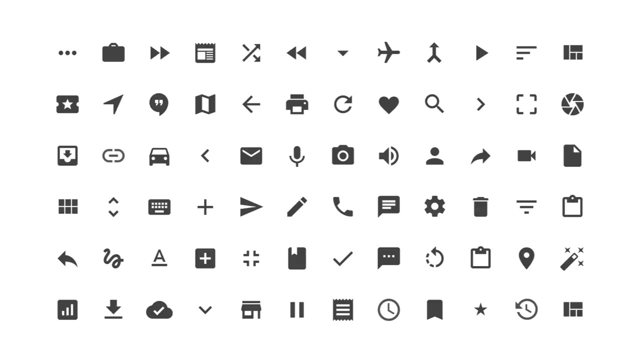 approach from app icons And applied it to the UI icons you see in your app. Our design teams are now using one common set of icons between Android, L, Polymer and the web. This means one trash can across all devices And we'll be releasing these icons later this summer. 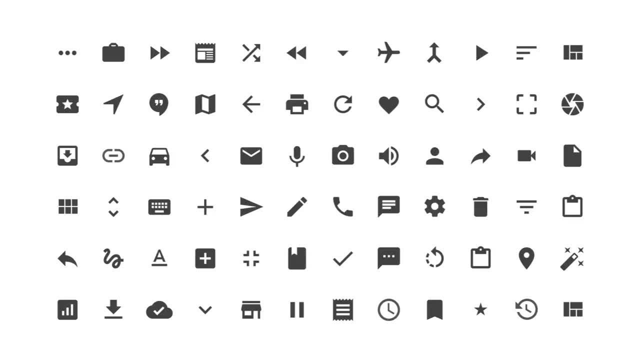 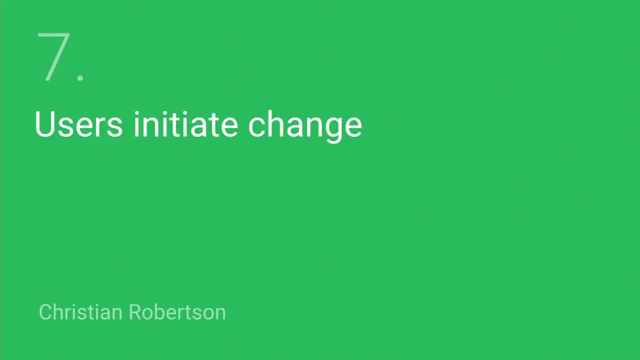 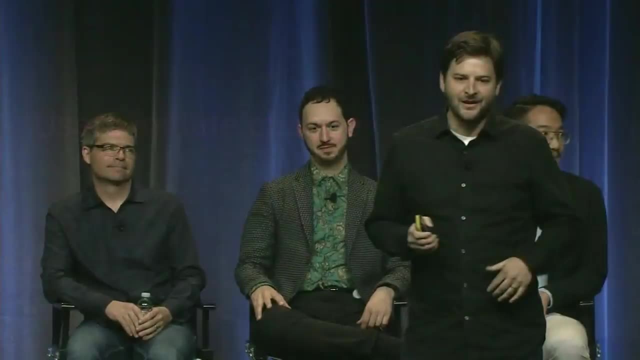 through our design guidelines, available for use on both Android and the web. All right. so even if we're doing all this and we've got great typography As an industry, we're leveling up when we start using baseline grids. We've got amazing color. 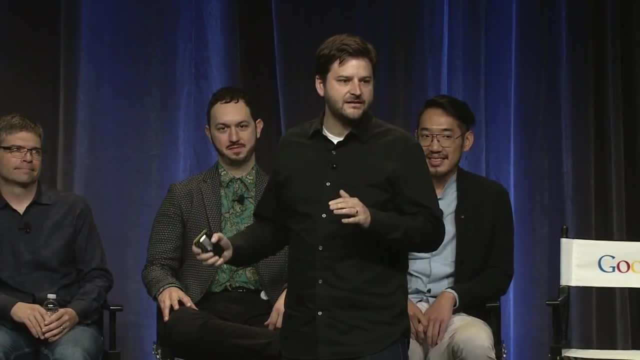 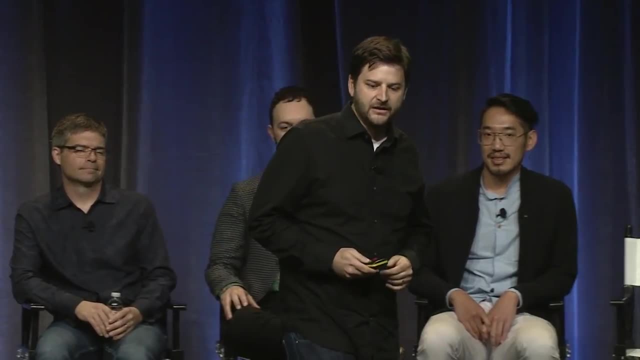 It's not enough just to draw the static states and stop there. We can do more to show people how the states are changing, letting them focus on the content that matters. So, when you think about it, almost all state changes in a UI start with user input. 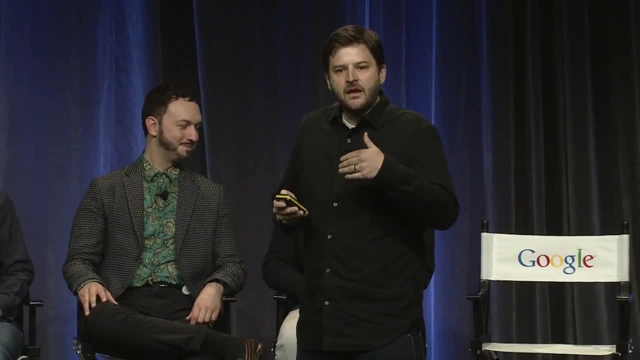 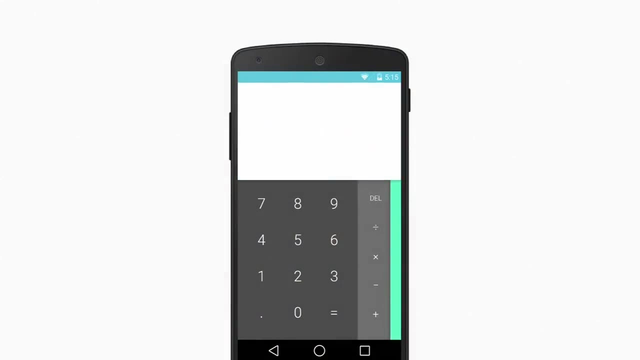 And this is why Material UI puts that user input at the center of the animation story. So when I touch the screen, immediately the surface changes, The surface responds. I can see exactly where I touched and the intersection of the object that's responding. 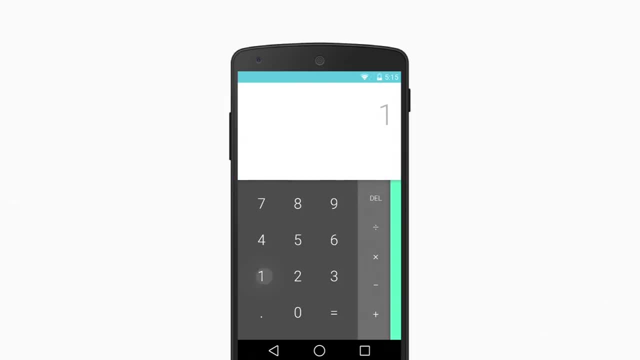 This does two things. First, it tells people that they've been heard, They feel powerful, They feel like they're in control. Apps feel responsive. Second, it confirms to them that the UI is going to do the thing that they expected, that it's. 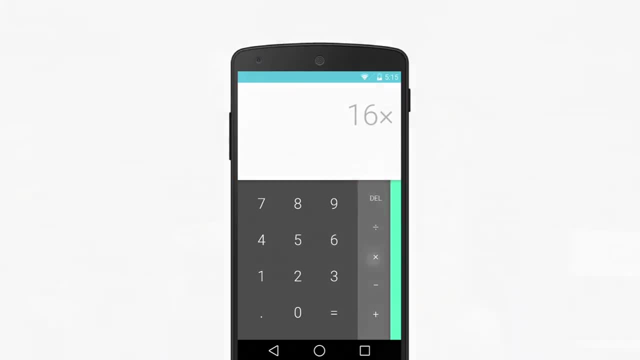 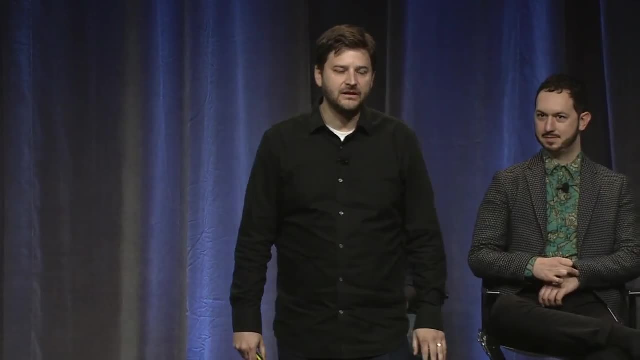 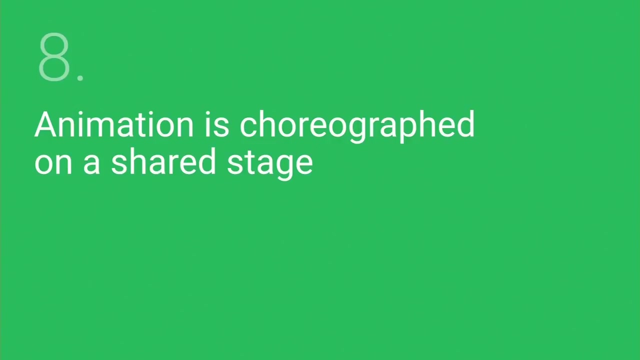 working. This animated touch feedback is now built into the platforms for both Android and Polymer, And it's being used by all of the relevant users. So it's not just the immediate touch feedback, though, that's centered on user input. The material itself transforms to bring in new content. 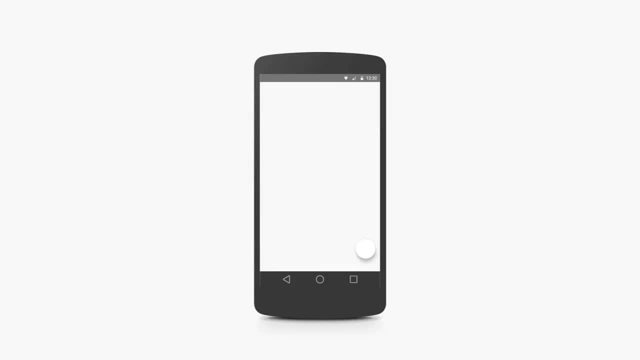 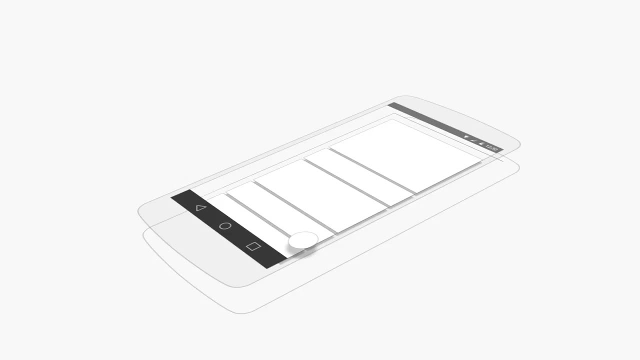 And all of this happens on a shared stage, And when I say a shared stage, I'm talking about the environment where this material lives. It's important to know, as we're looking at the material, that it lives in the same scale and in the same space as we do. 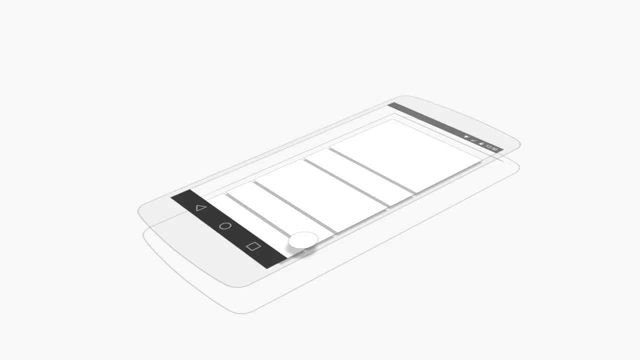 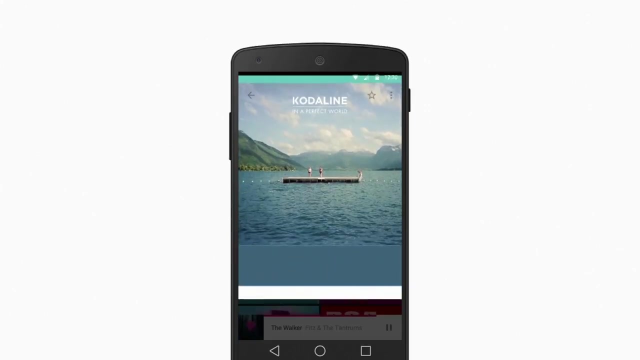 We're not flying through some imagined space or looking through a window into another world. This material lives in the same scale as the device itself, whether it's in our hand or we're looking at it on our desk, We don't move The material does to bring the content to us. 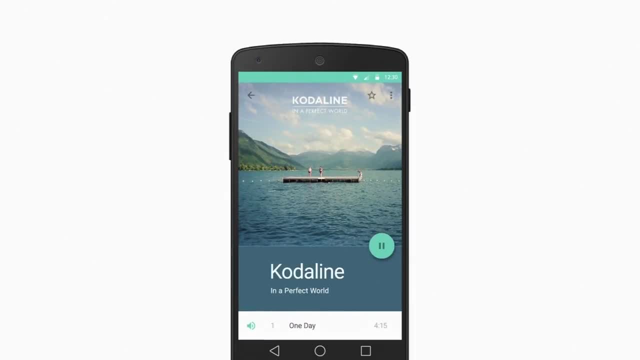 You can see how this works: as transitions organize themselves around the object as it's selected, The material moves, expands to reveal the new content And notice that even as the content transforms in a way that maybe a physical material like paper wouldn't. 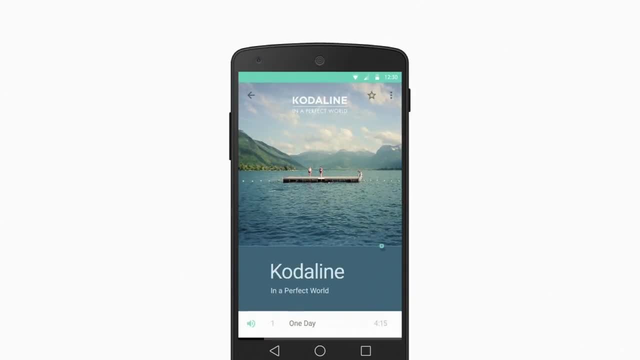 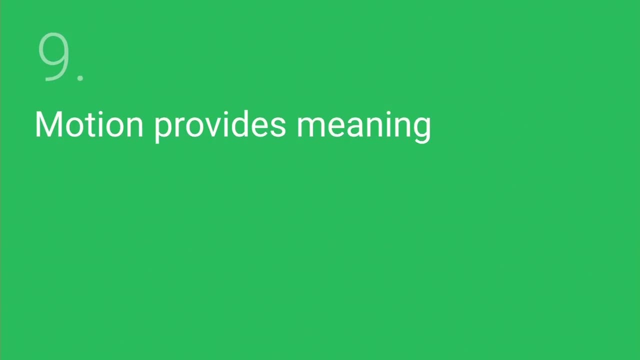 it's still very clear what's happening because of the way the material responds to light and the way the shadows are being rendered by the platform. So animation is crucial to reinforcing this metaphor that Matias talked about. It's just in the same way that the shadow rendering helps. 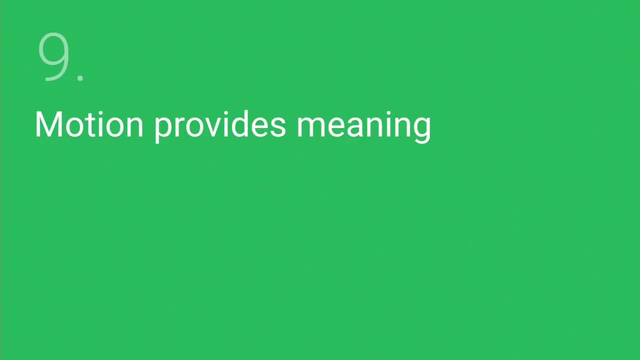 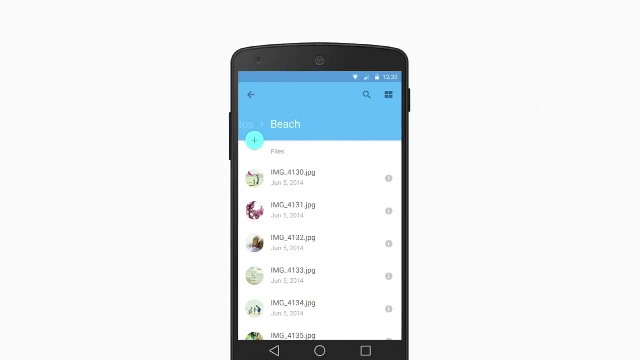 us understand what we're looking at. the way that things move give cues about how they work and about their properties. So, for example, the material animations naturally show continuity from one state to another. When I select an item, it expands to the next state. 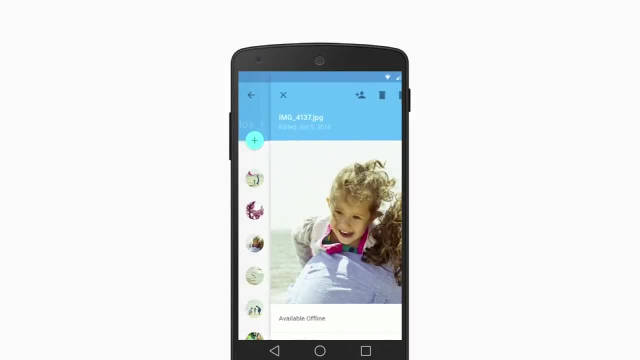 It doesn't jump cut, It doesn't blink in and out. It moves naturally, like sliding a piece of paper across the table. If we teleport our users from one state to another in a UI, it can be confusing and disorienting when they get to the other side. 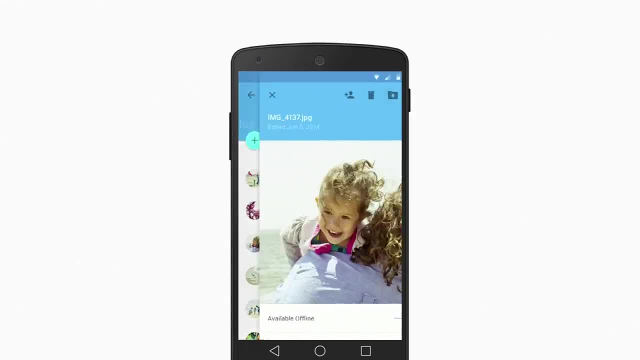 Almost like if we were to be teleported in the real world. if I were to just appear on the stage in front of everybody here, it'd take me a few moments to get my bearings. It's the constraints that are inherent in the material that 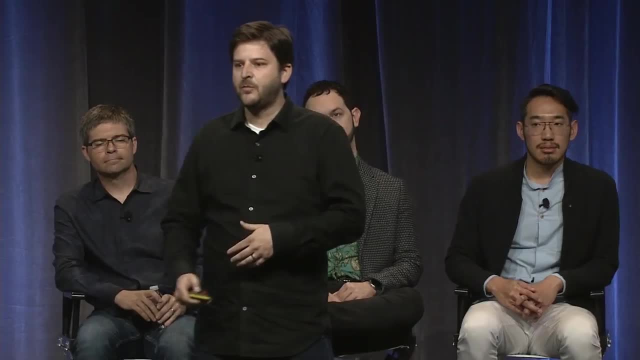 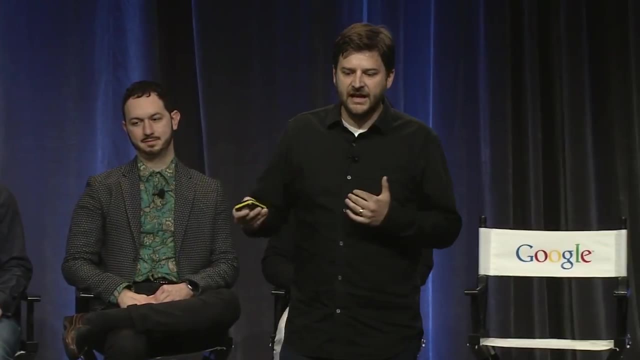 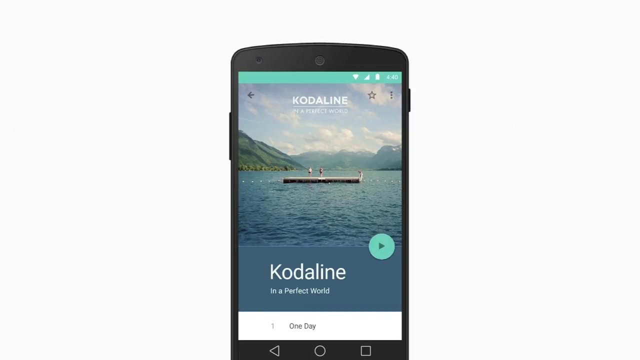 make it clear for people what can happen, and it lets them predict and understand what has happened. So, if it makes it easier to understand what's changing, at the same time it can show us what's important. So, since our eyes are naturally drawn to motion, 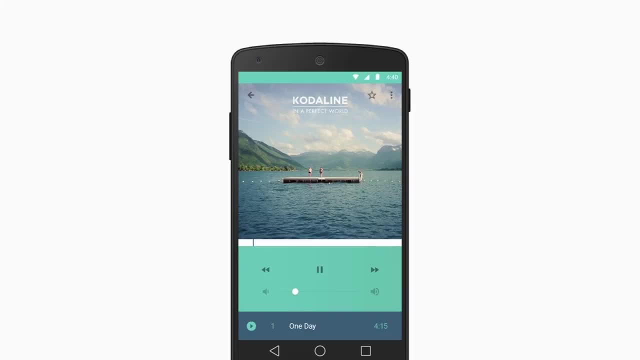 if something moves and it's in our field of view, we're going to see it. It's a really strong tool for us to help direct focus. If in a music screen, the player controls are the primary interaction, the animation can point that out. 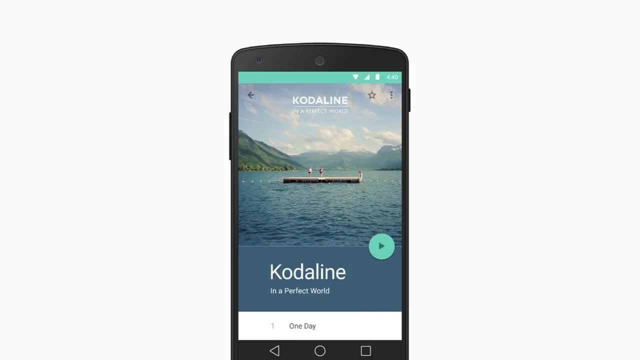 Also even noticing the details, those small things that you might not even notice overtly, like, for example, the small slide on the screen, On the control slider as it comes in. Wait for it. There it is. Even though people might not notice it overtly, they see it. 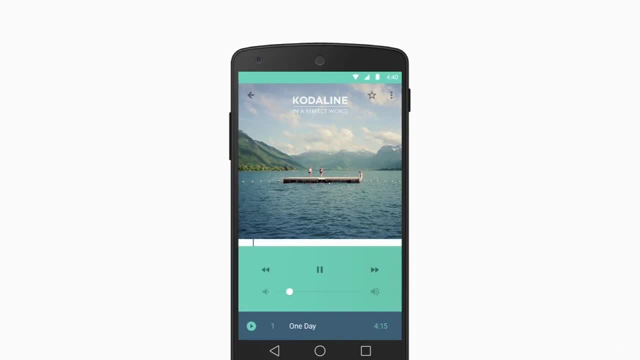 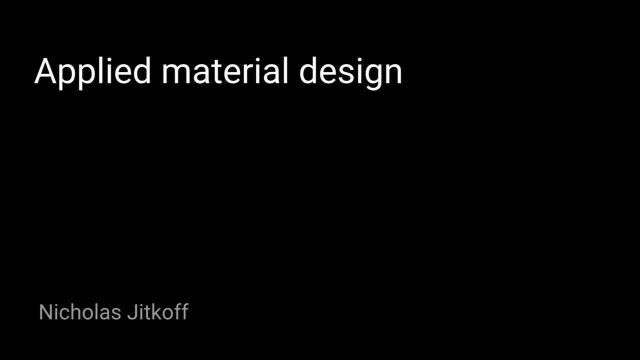 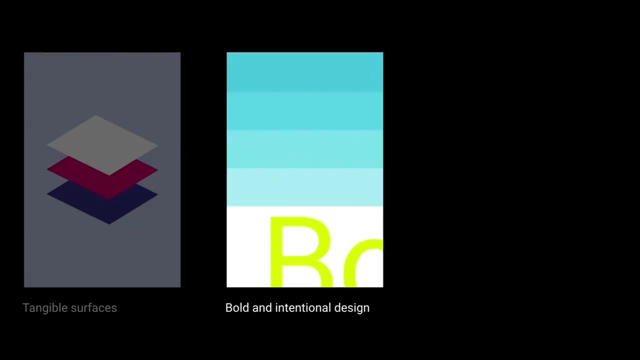 and they know how things work without having to think a lot about it. So these guys talked about many of our core principles. primarily, the sense of tangible surfaces which appeal to the primal parts of our minds with dimension and shading. The second, the concept of design. 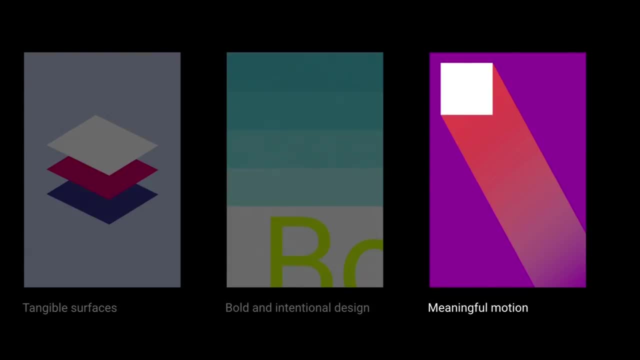 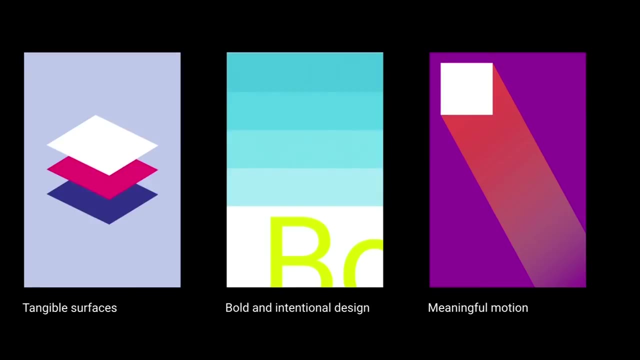 It's a very powerful concept that involves an intentional design which provides a unified language that allows brand and UI elements to stand out, And meaningful motion, which fuses this design and the surfaces together and gives new affordances and life to UI. 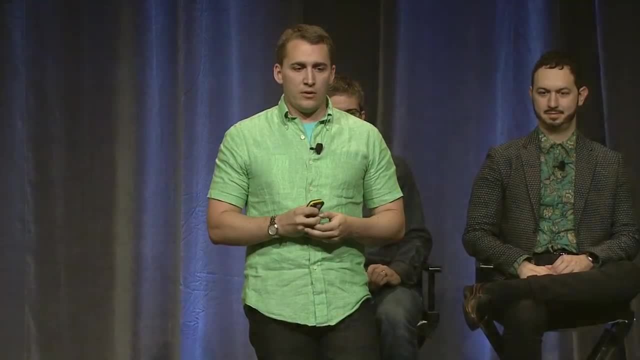 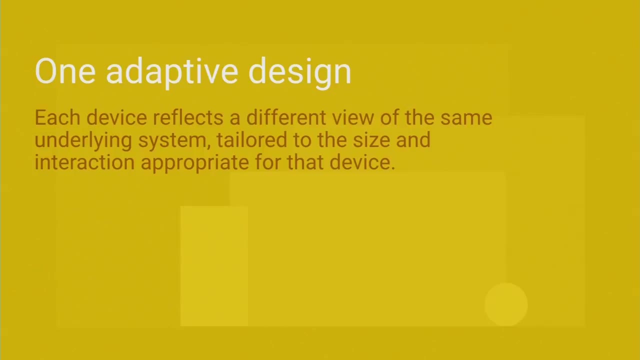 What we want to use these for is to create a new unified experience for users. We're surrounded by devices, and people experience our work across all of these different platforms. For that reason, we want to treat every device as a window on the same content. 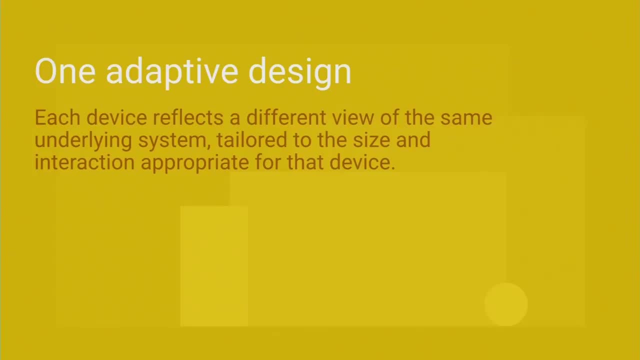 We want to tailor the form factor so that each one of them has commonalities but also can be unique. Color, type and spatial relationships help tie them together. In this example email app, the sizes are all related by color and structure. 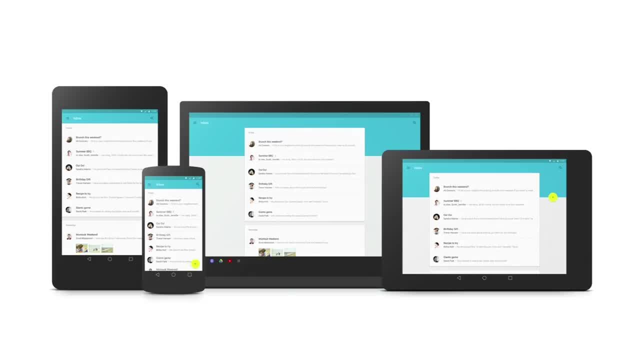 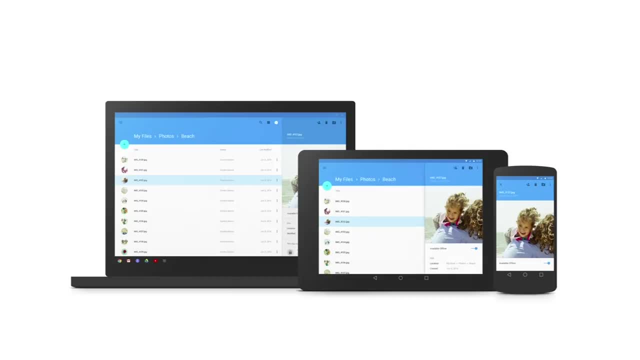 But there's diversity in the overall presentation. The larger ones use cards so that line length is kept reasonable, And the small ones end up being full bleeds so they can take advantage of the size of the device. In this files app there's a drawer on the side. 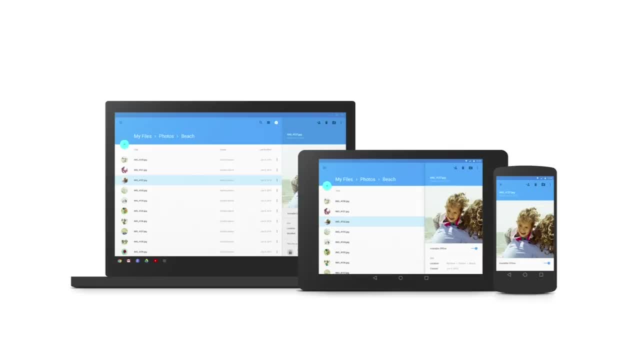 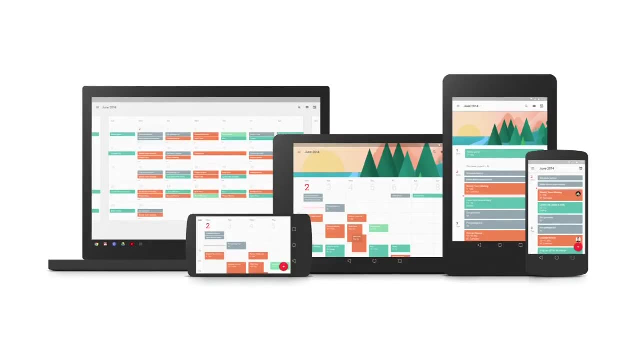 But on desktop it becomes a persistent element. On tablets it's a temporary overlay, so it stays out of the way, And on phones it's a persistent UI that you drill into. In this calendar example there's more variety between the views. 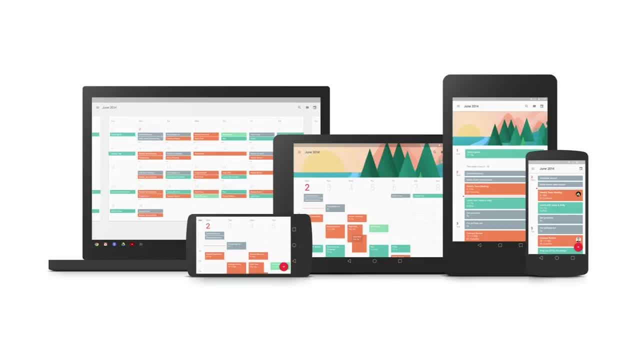 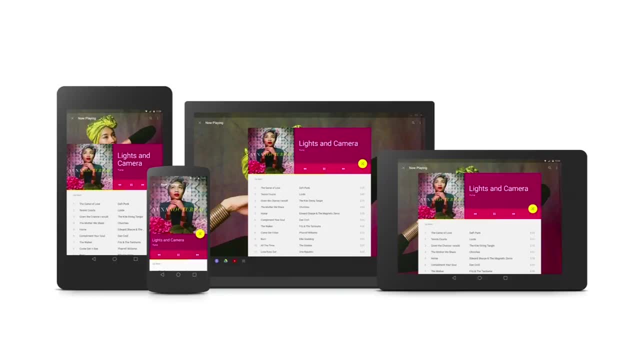 But again, typography and color tie them together, so they feel like they're a consistent experience. Immersive imagery also plays a pretty big role. This is something we've seen on mobile, where people are doing things full bleed that we actually want to take back to desktop. 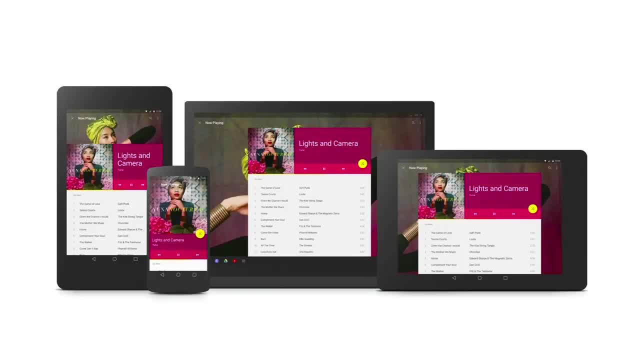 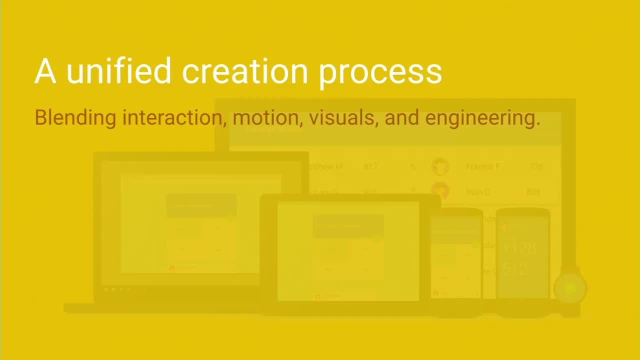 It looks great there as well, And in particular when things used to be sort of full bleed. we now can use things like cards to keep that same sense, even though they're now surrounded by other kinds of content. Beyond the platforms, we also care about working. 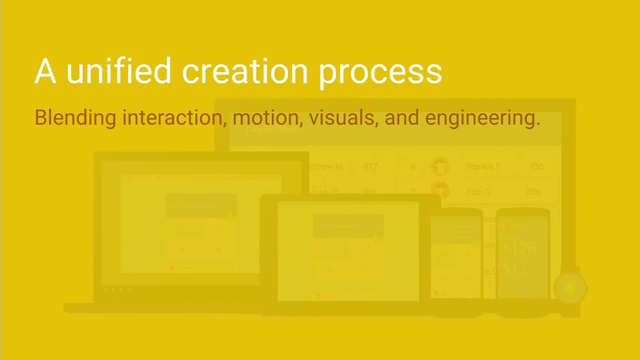 with different disciplines. Interaction, motion, visual design and engineering are often not deeply associated, And so we've been using this material metaphor as a way to bind the different disciplines together and make them more collaborative. In interaction. the materials reinforce the overall sense. 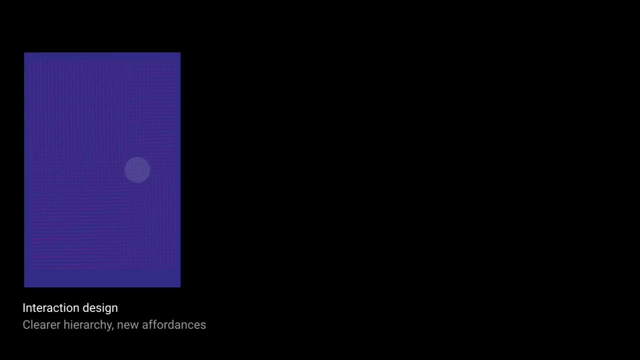 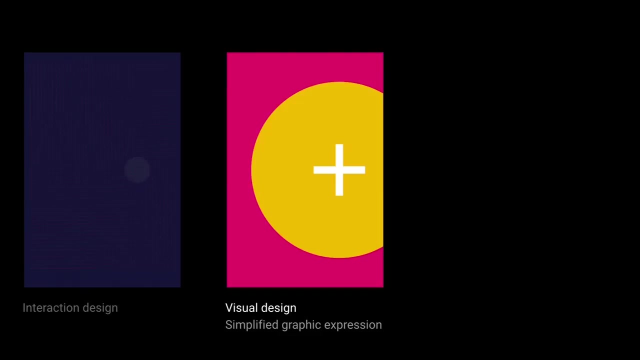 of hierarchy. The scrolling and layering give a good sense of how gestures work and emphasize how the user should focus their attention. Visual design becomes simpler because of this. The content itself can be very graphic in its hierarchy and rely on dimensionality for higher level structures. 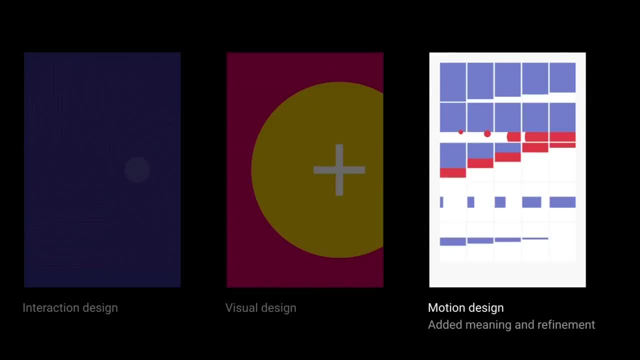 like toolbars or other elements, so they're not considered together. And emotion is in most ways, the most important. Materiality provides the grounding for it. It makes it consistent and intuitive, so it's obeying realistic physics and speaking better to the user through that. 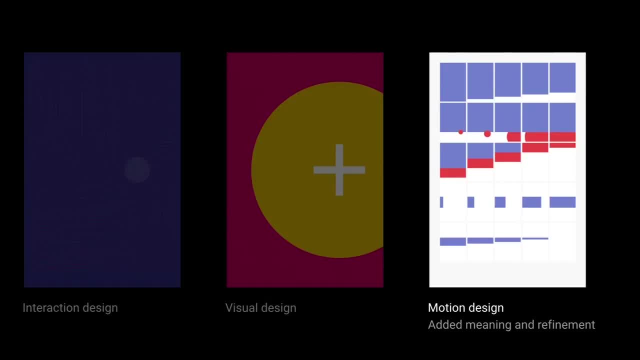 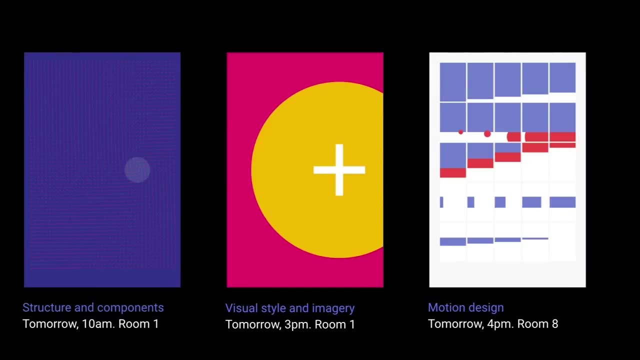 More importantly, it allows motion to be deeply tied into interaction and visual design. We've got sessions tomorrow and we'll talk a lot more about the interaction between these different elements, starting in the morning with interaction design and then in the afternoon with the visual design. 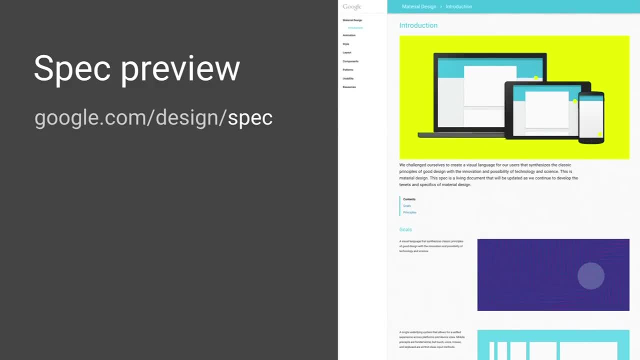 If you're interested in learning more now, you can take a look at the initial spec preview that we put up. There's probably more than you're interested in seeing in the moment, but you should come by and listen to the talks. We'll point out the most important parts. 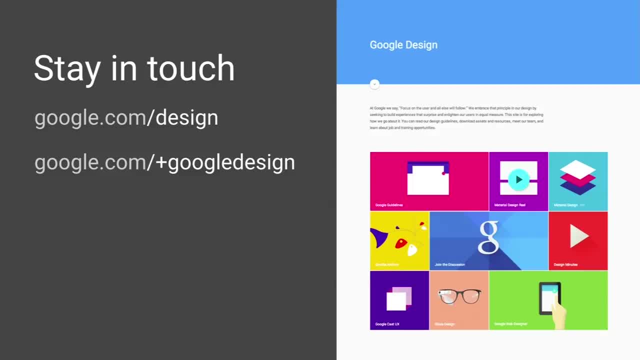 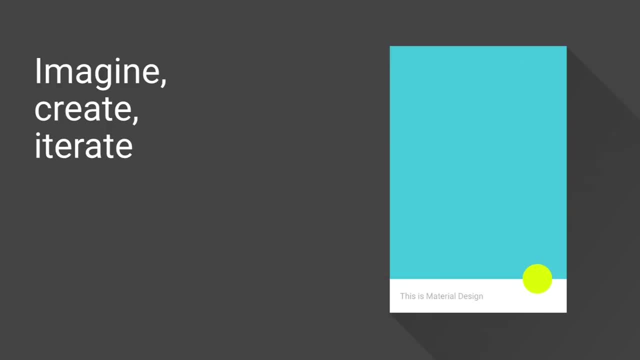 And stay in touch with us. We put up a new site for googlecom slash design, as well as a plus community, so be sure and follow us there. We created these principles as a tool for all your future work. We want to inspire and involve your designs and your apps. 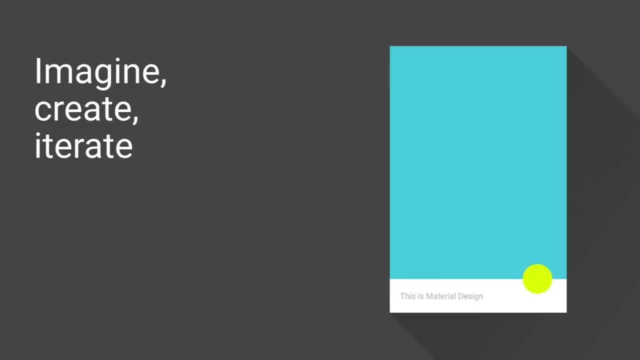 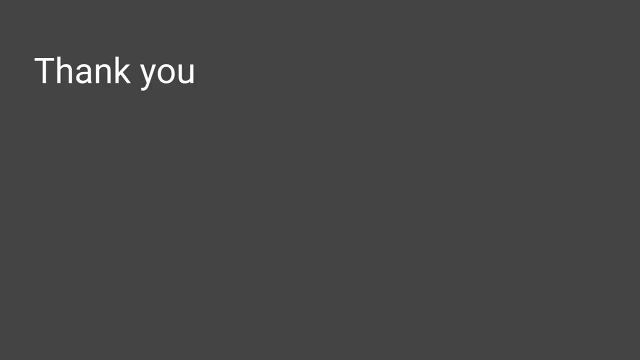 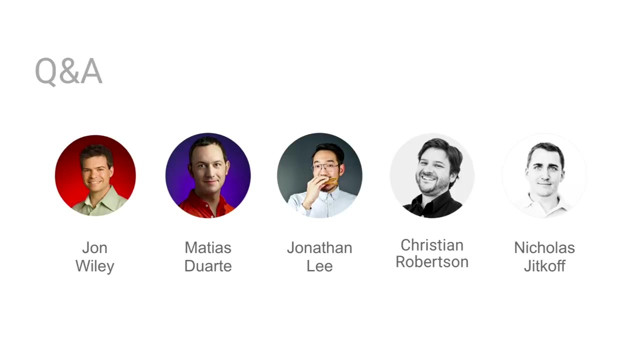 So, in addition to these sessions, we'll have a number of Design Sandbox events. You should come by and talk to us, But thank you for joining us. So we've left time for questions And there's actually microphones in the center aisle here. 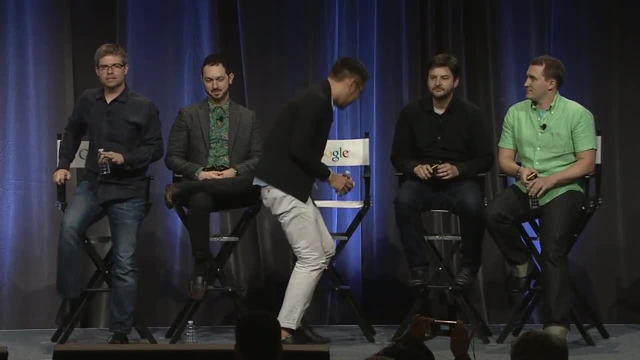 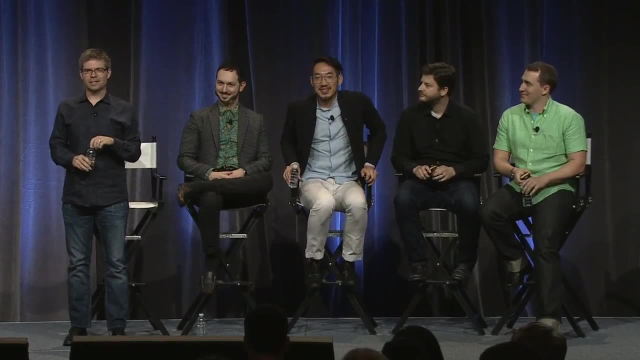 There's two: There's one in the back and there's one up here. So if you all have any questions about this or design at Google, or Nobody has any questions, Everybody just wants to play with cardboard. By the way, if you've tried the Google Earth on the cardboard, 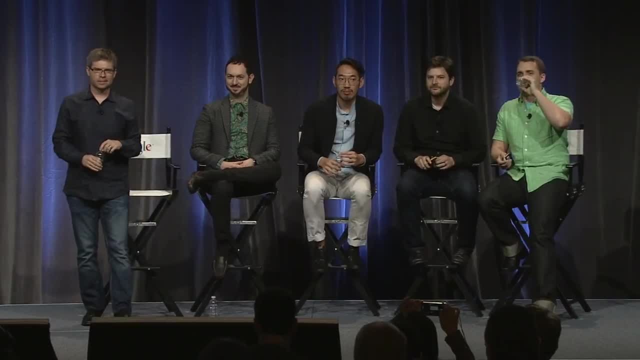 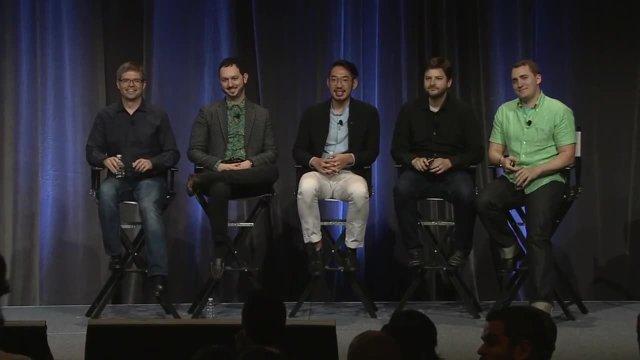 thing. it's just amazing. Here's a question. I apologize, I'm a developer, not a designer, So this is a silly question. I like design, though I see a lot of circles. What's up with the circles? 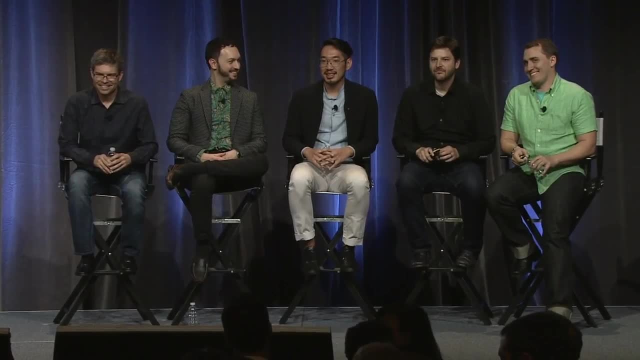 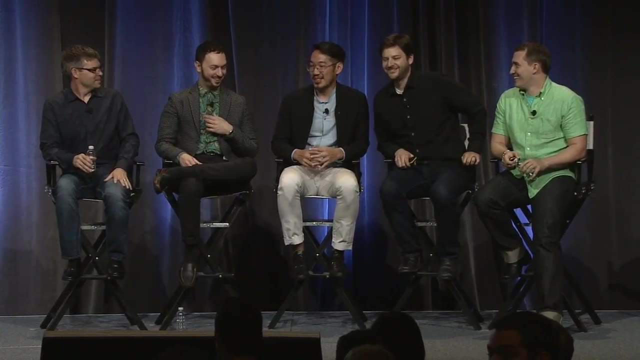 I like them. I like them, Just could you speak about where they're appropriate, what you see them conveying to the users, stuff like that Circles. Who's going to take the circle question? Matthias takes the circle question. Oh, OK. 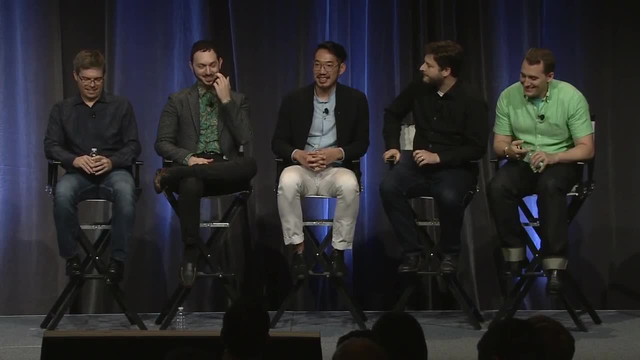 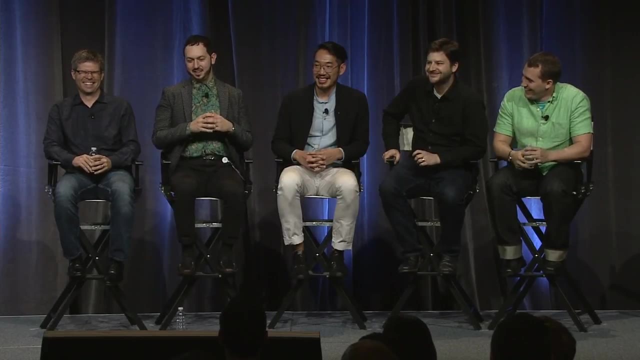 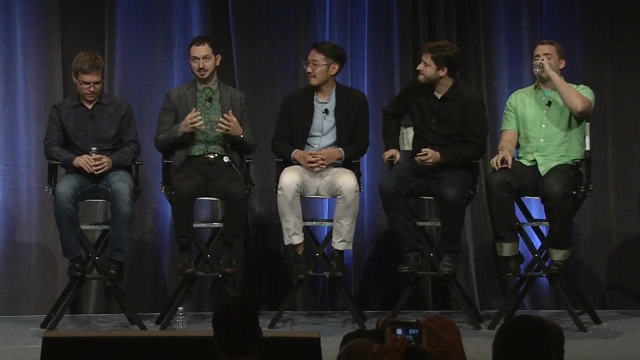 I'll take the circle question. I really would have thought the circle question should have belonged to the art directors, But so one of the things that the circles provide. well, there's a couple different ways that we're using circles. Actually, it's probably good to step back and talk about one. 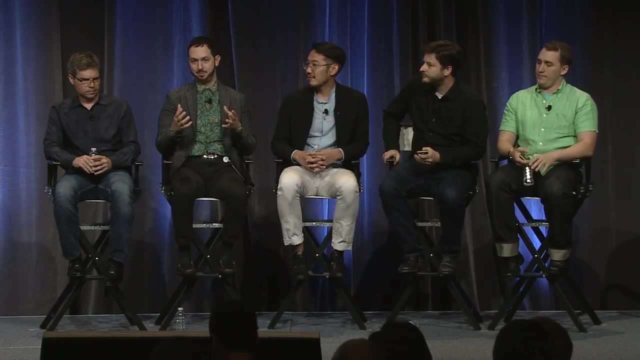 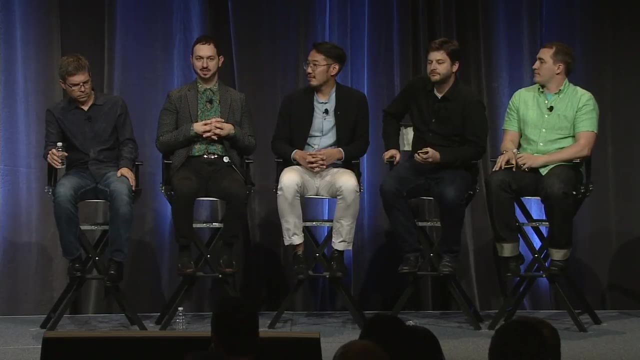 of the ways that we've simplified and we've tried, But one of the ways that we've tried to keep very low level and elemental and primal. what we're doing in material design is everything is really its most simple and basic geometric shape. So you'll see circles. 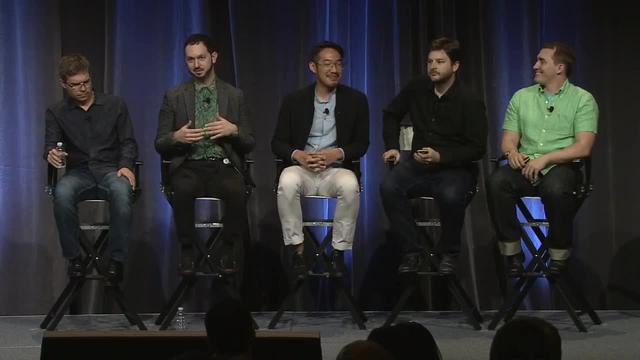 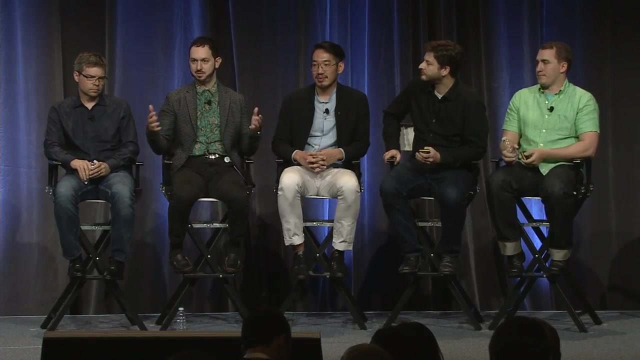 You'll see squares, You'll see rectangles, You'll see, basically, divisions of space. So when you want to have a contained element, the simplest way to do that is to bring in the circle. So we use the circle Because it naturally has contrast to a space. 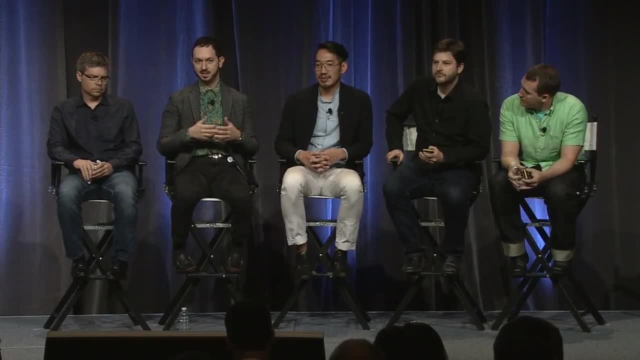 that you've divided up and that has blocks of text or areas that have been created by cards or divisions of color. the circle is a great way to draw your eye, without motion, to those elements that you want to emphasize, whether that is the floating action buttons, that 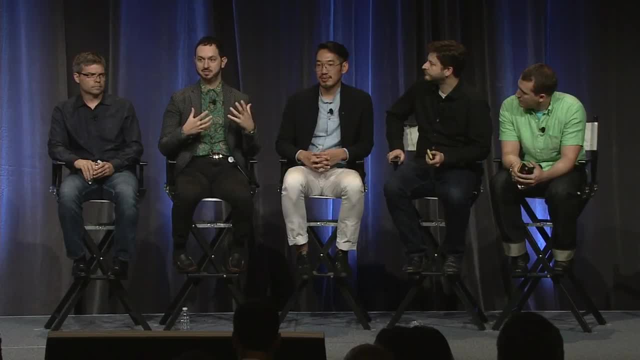 are indicating primary actions or it's the avatars of people that are very important. Circles create rhythms themselves that help you organize and scan, Scan through the page, like when we have the multiple messages and email. So the circle, what you should think of the circle as 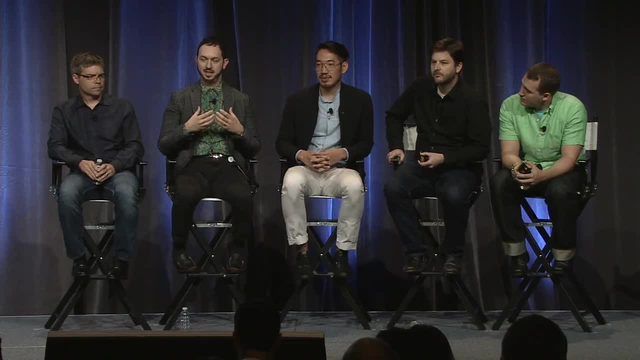 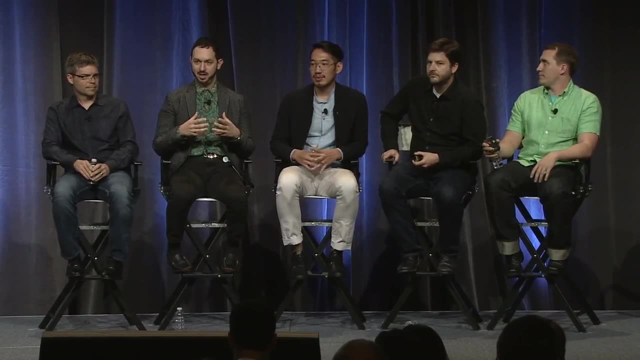 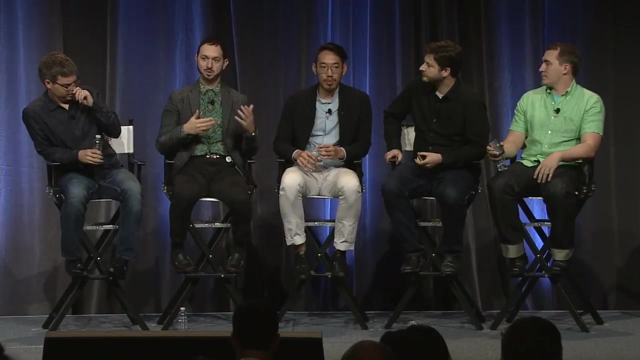 is. it is an element, a geometric element, that is a visual design tool. like any of the other tools, It, perhaps in a very simplified shape palette, stands out, And that is its attribute: that it does stand out and you want to use it in places where you want to stand out. 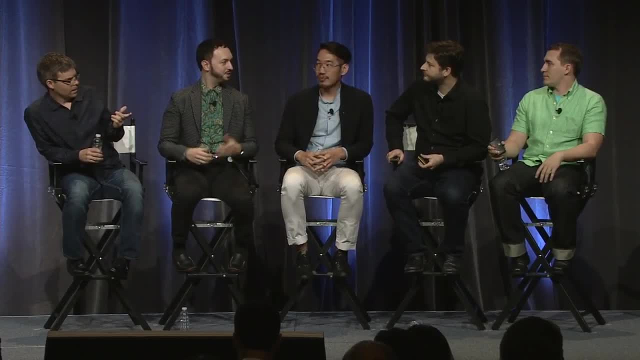 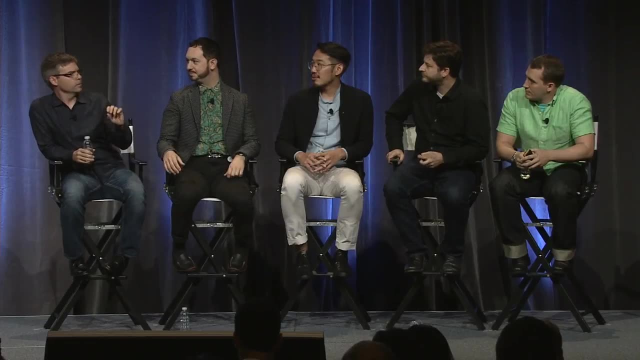 or you want to create rhythms by repeating it. Did you guys want to add anything to that? Yeah, I was thinking about sort of where a lot of the circles kind of came from and kind of how we in the early days when we were thinking about this- 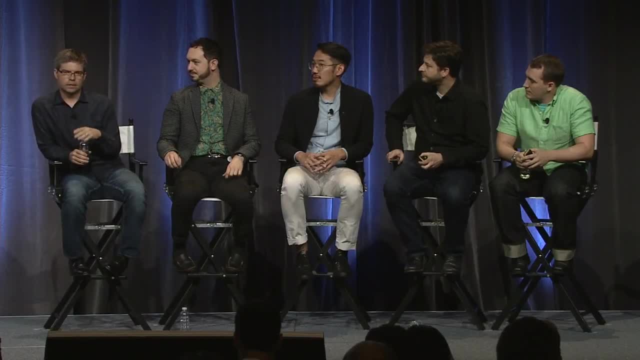 So at the beginning I talked a little bit about its material principles and the underlying physics, And one of the things that happens with any interface, if you're interacting with it, is you're injecting energy. There's events that are happening. You're either interacting with it. 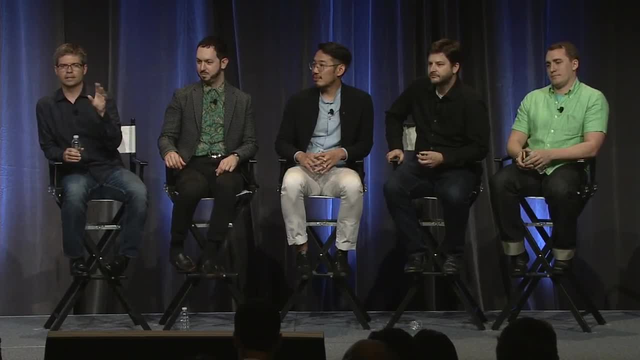 you're touching the interface And you're sort of as you're using it, you're injecting energy into the process of things that are happening, And one of the most fundamental things that happens within physics is that whenever a signal happens, whether it's sound or light or what have you- 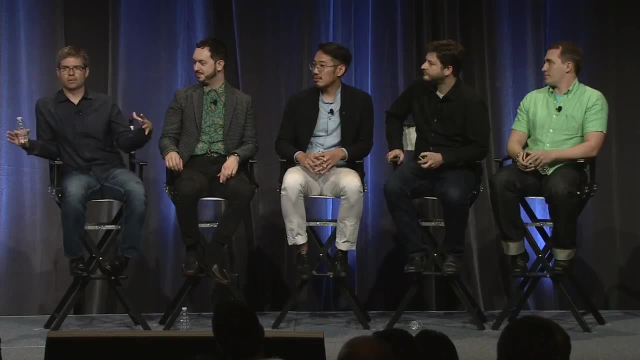 it propagates in a circle. It propagates from its point of origin and ideally at the same velocity outwards, And that's generally in a sphere, in a constrained depth environment. that's going to be in a circle. And so when you see not only the circles in terms 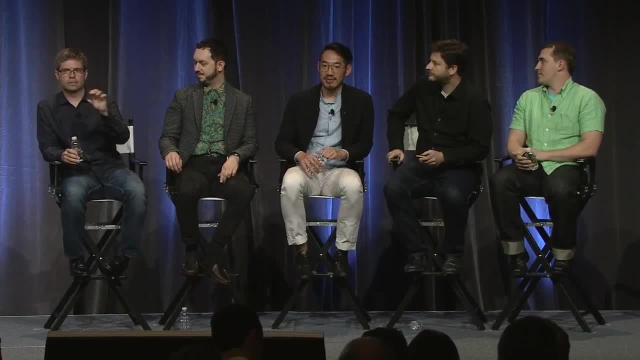 of the affordance for interacting, but also as you tap on things and that circle radiates. it's really about just conveying the sense of the physicality, the energy going into the system and that that's actually your actions, or spreading forth into communicating with the rest. 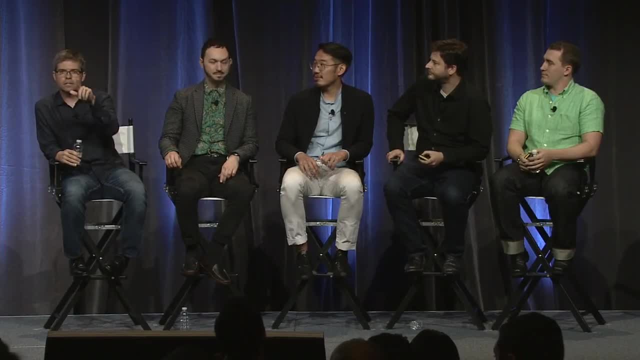 of the things that are on the screen? Next question: Yes, My question is regarding the form factor. It seems like it's the apps. now, with the material, you'll be able to design one app and basically the app will adapt. It will be responsive to the screen size that the app is running. 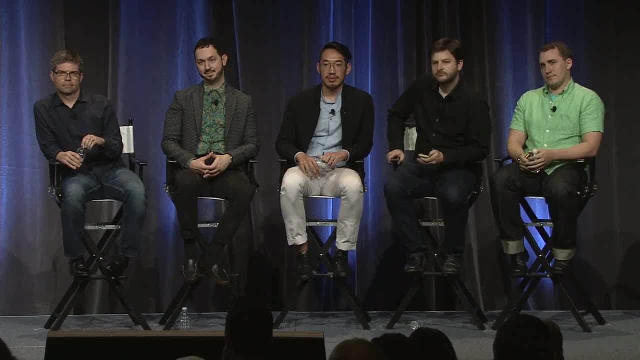 Is this where this is going, Where, with the material, you'll be able to create one code base and be able to run the app on any screen size. Do you want to talk to that one, Nicholas? Yeah, So there's two sides of this. 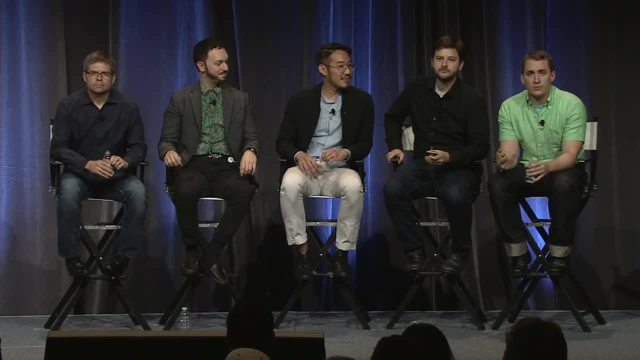 One is: we want to make it as easy as possible to not just reflow to different sizes, but also to tailor the way that we reflow in a unique way. So, while the default platform behavior will do the right thing as far as allowing you to expand, 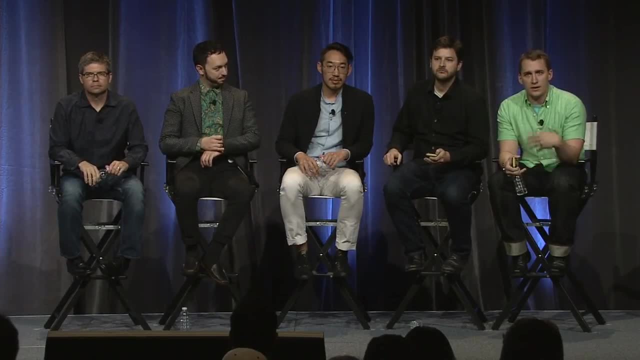 expand things to different sizes. we do want more thought and attention placed on how it should actually accomplish that. Beyond that, a lot of these design guidelines are intended to make that much more seamless of a transition, like the commonality of iconography and typography. 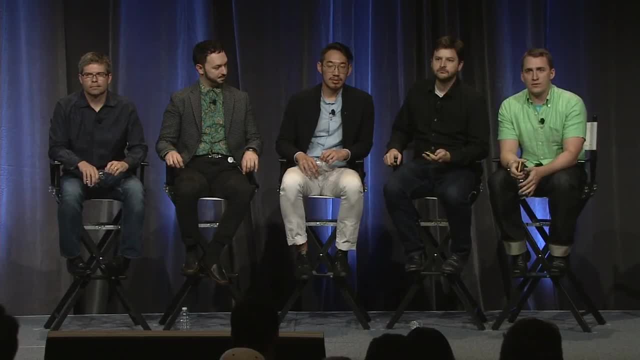 those, blend them together even as we introduce more differences. But our prime focus right now is trying to get these things to carry a design across those different form factors. Yeah, I mean I'll be a little more explicit as well. I mean, for starters, we do have two code bases: one if you're developing native apps for Android and one if you're developing with Polymer for the web. There are framework components in both apps which will make it easier for you to scale between different screen sizes, But there is a lot of intentionality and design thought. 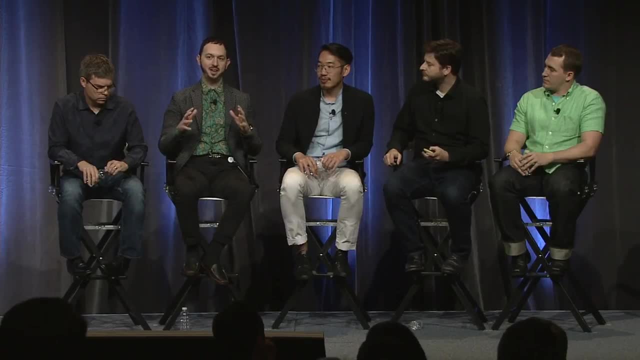 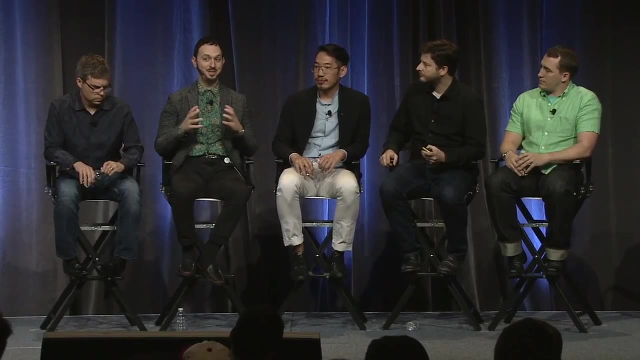 that needs to go into making some of those decisions, So we don't have one automatic system that will take any application and automatically scale it for you to any screen size. Yeah, I mean, I think that's something that we're trying to do. 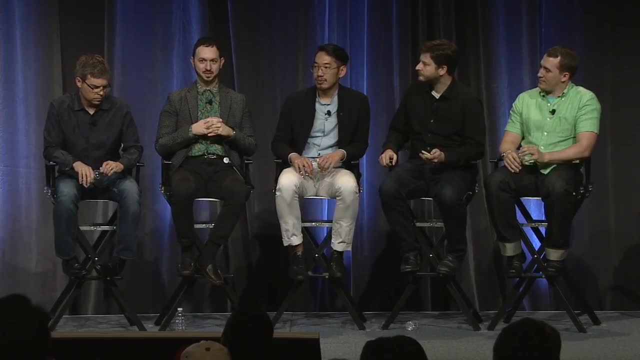 Maybe someday, but I think that would actually require intelligence that's pretty close to that of a developer and a designer combined. What we do have here is a design system where you can create a coherent app and use the same design and have very straightforward ways to adapt it. 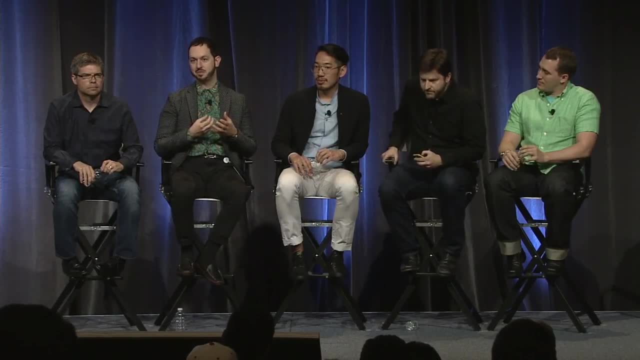 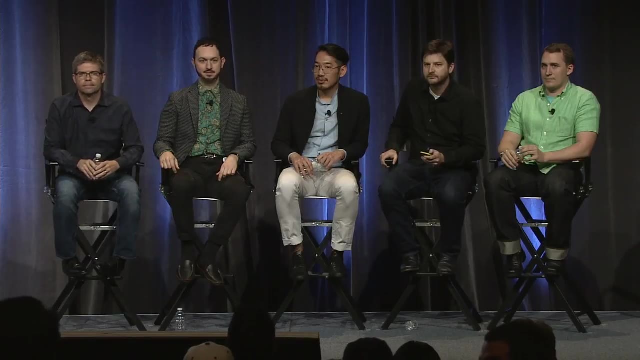 if you understand also what the purpose of the app is and what is appropriate for the different screen sizes. And that still requires a human Cool Next. By the way, I guess all the line is: yeah, OK, great, Yeah, you're good, you're good. 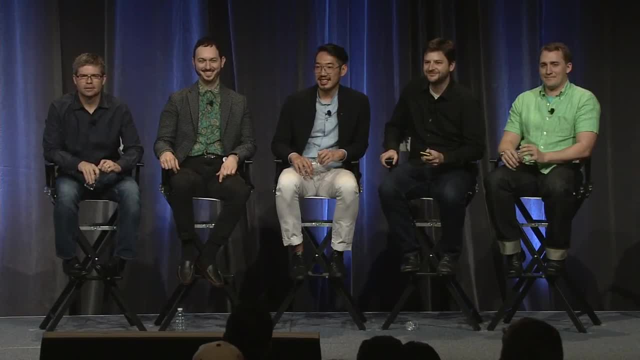 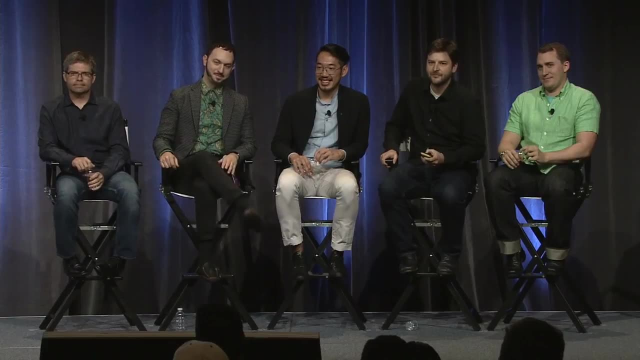 First off, you guys rock. Thank you, Yep. So I'm a big fan of the animations and giving cues and to the user and everything, But sometimes it could be too much, right? So at what point do you say you know if I hit the play button? 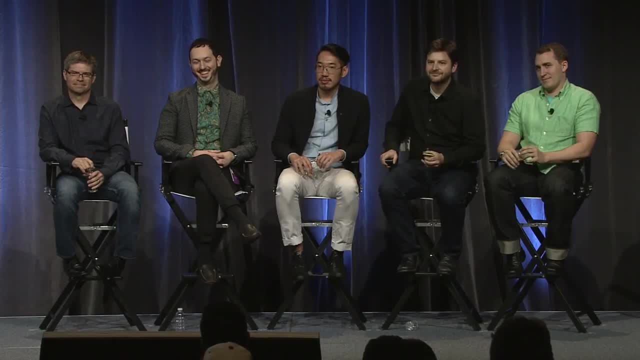 it's going to go around the screen three times, come back in and pop it, And it's going to pop up Because some users can't. It happens on every press, every single time, So sometimes users can see that as a bug. 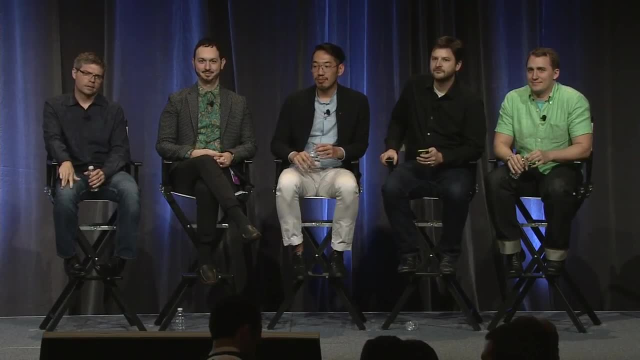 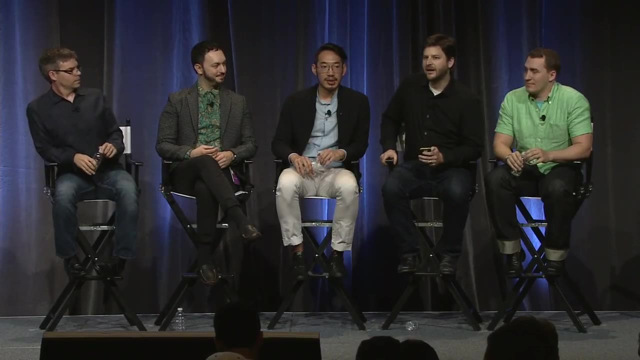 or it might slow them down to whatever actions they're doing. So were there any concerns around that And, if so, how do you tackle that challenge? Yeah, so I think one of the things to know about this isn't just true of motion design. 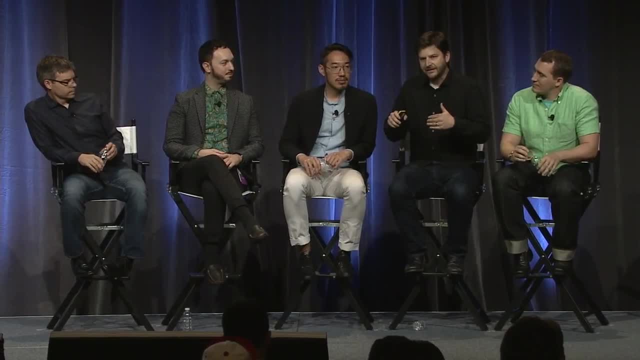 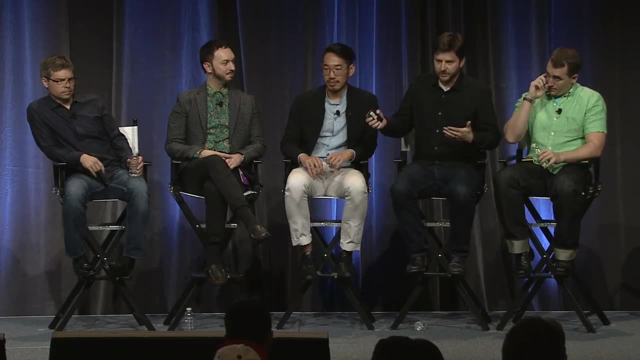 it's true of design generally that there's a lot that's going on below what people notice. So we don't actually want people all the time thinking about the animations when they're going from one state to another. We don't want them to say, gee whiz, I just opened up that email. 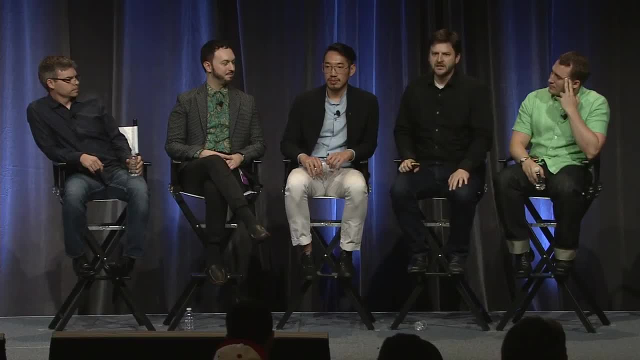 And again I saw that animation. We want them thinking about the email, And so if you apply that standard- as how much do I want people thinking about the animation themselves, What is it trying to communicate? Then you can kind of back it down to the right level. 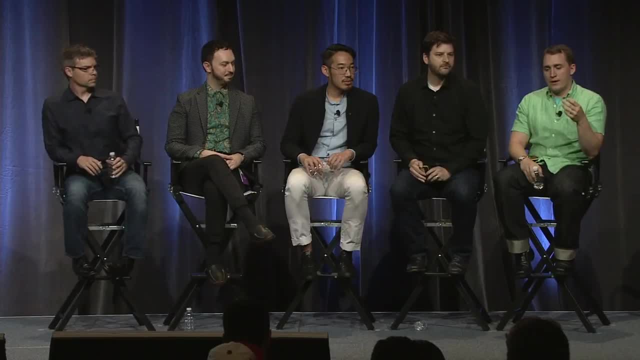 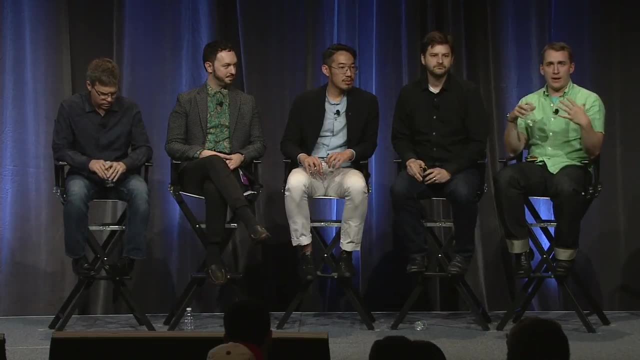 One of the things that we considered consistently throughout this process was how to use the animation to sort of go along with the user's intention. Yeah, Because when you have touch responses that sort of emanate outwards, it's very easy to hide details in there that reinforce what's happening. 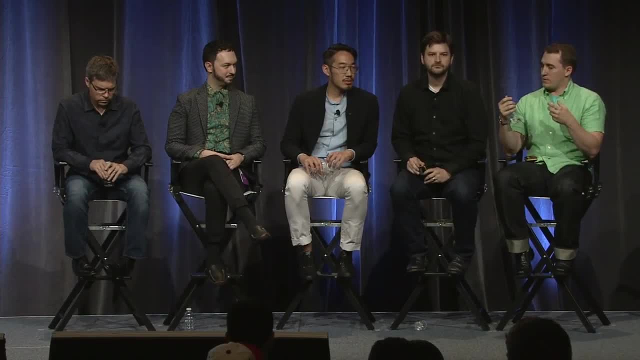 without feeling like you've added a bunch of animation in there. So we'll go into this a bit more tomorrow. But having things sort of move counter to the direction the user's doing things draw attention to them, And if you're going to do so, you should do that intentionally. 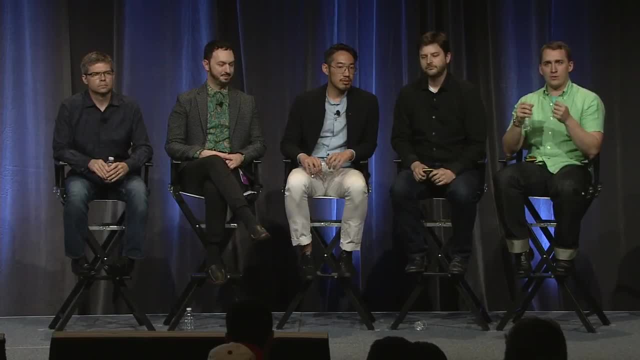 If you don't want attention drawn to things, there's places to hide them, And it's really about trying to figure out how you want to balance it and where you want to draw people's attention. Hi, So I was wondering if you could extrapolate. 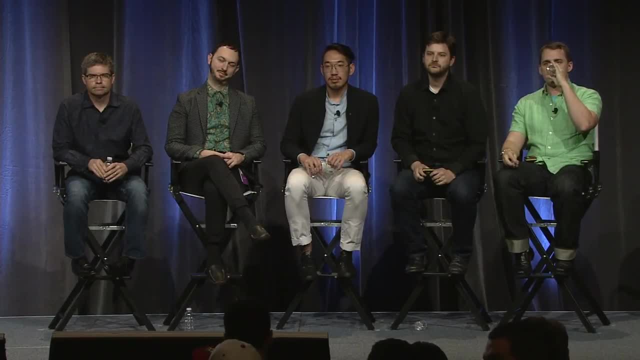 on how you see new forms of input with respect to motion. So, in regards to wearable devices, let's say a swipe left and a swipe right with a wristwatch or drawing a circle in the air- how would that integrate with the user experience on an app level? 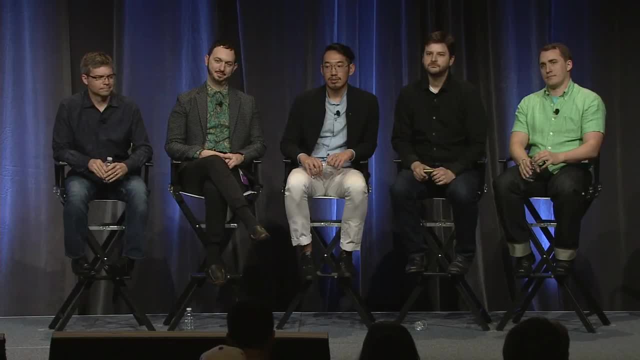 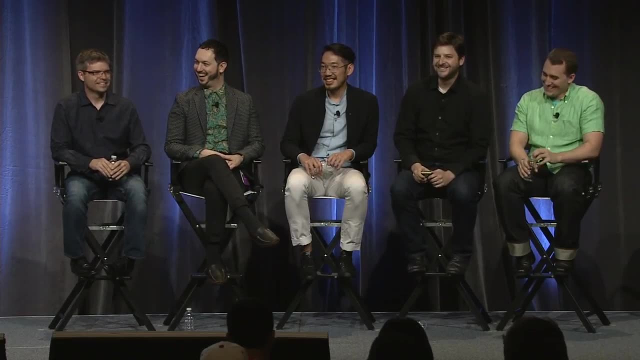 let's say, or on your desktop, And how that would sort of integrate. We've been getting, We've been given a design challenge on the fly: How to design gestural interfaces. I think a lot of this, I think, goes back. 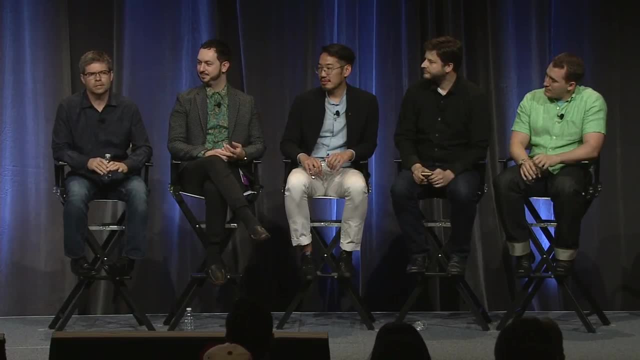 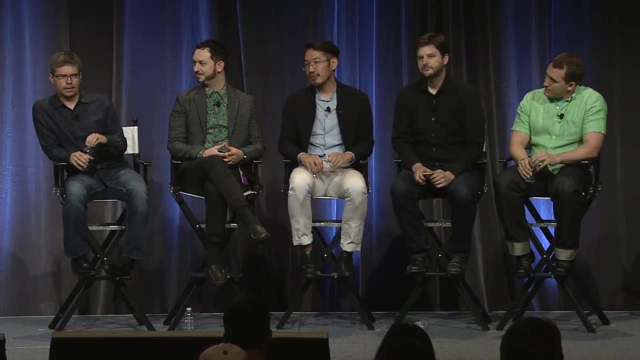 to the material as a metaphor, And part of what we're trying to do is you go and you watch summer blockbuster sci-fi movie And sometimes it can be a little bit of a letdown because they set up the world in which they're operating. 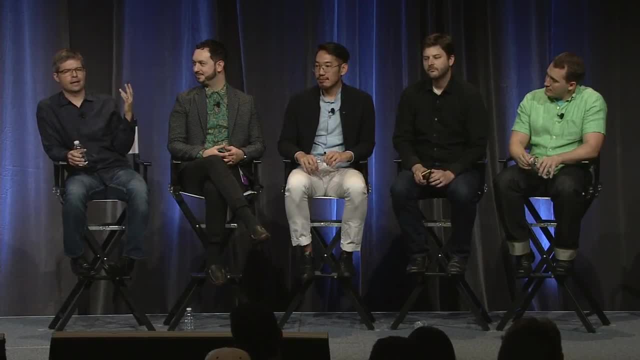 but then they break some principle right And it just kind of falls flat. Why did that happen? I think part of what we're trying to do with a system like this is to set up a series of sort of a world in which it functions. 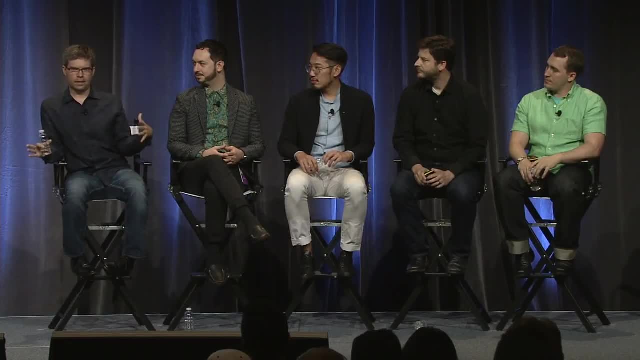 And ideally it's grounded enough in the reality that we have here, such that you can bring your intuition of how objects function to the system, And it fulfills those expectations and hopefully exceeds them. But then maybe we add an additional magical things that. 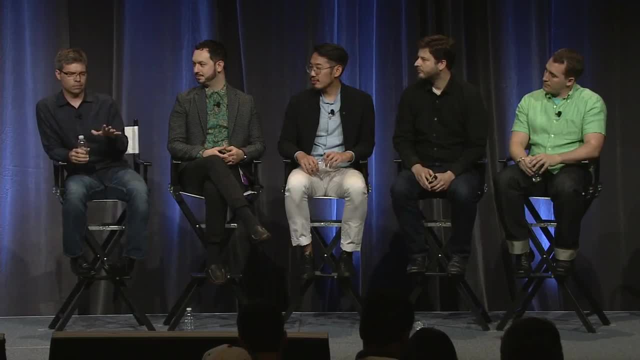 you know, can't. You know? we can't quite do yet with physical devices because we're rendering with virtual devices. The bridging of gesture and other types of interfaces to me is actually just another level of you know, it's another additional dimensionality. 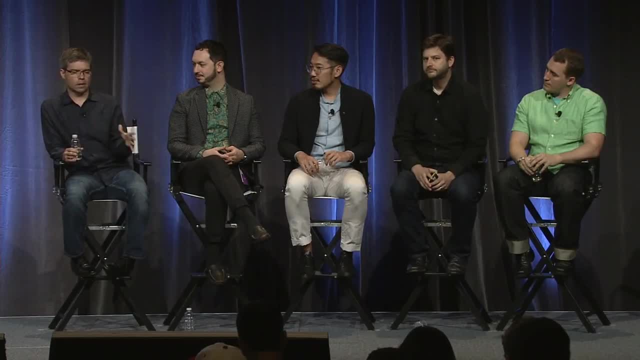 in terms of interaction And it's a progression. So when we started with computers, we basically had keyboards right And then it's like, oh, eventually we got a mouse, And so that was like a little bit of interaction slightly removed. 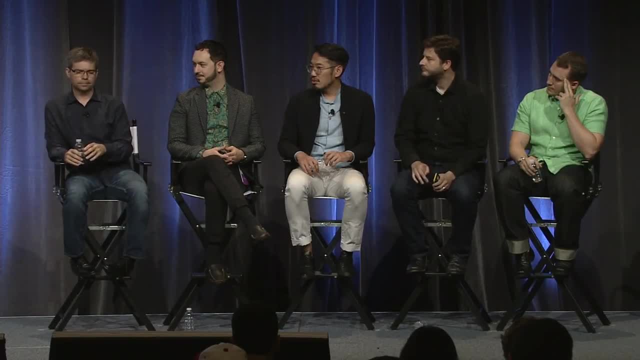 You know, here it's happening up here and I'm using these things to control it. And then we get all the way now to today, where we have smartphones with touchscreen displays, And so now we have this additional dimensionality of being able to physically touch the software. 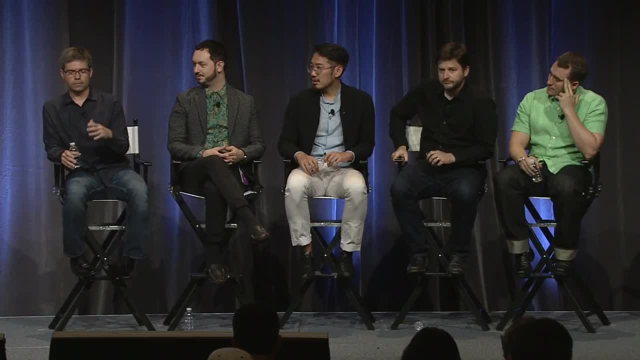 And now we're adding this other layer in, hopefully over time and hopefully do it right, where we have wearable devices that have gyros and stuff. I mean, even the cardboard device actually is really fascinating because, again, it's really awesome. 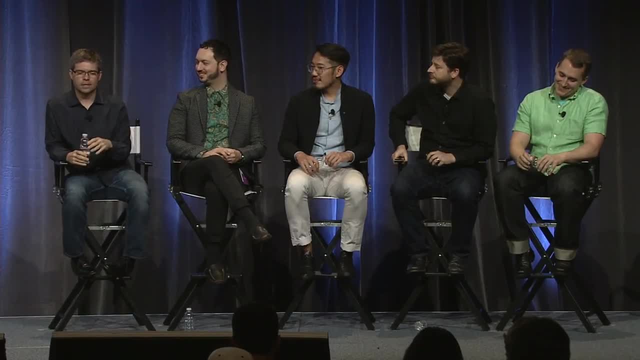 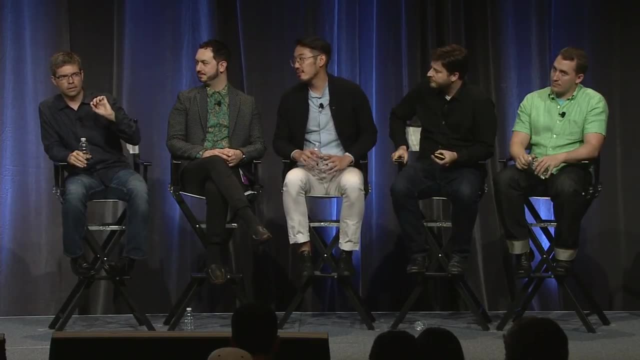 You play with it, But you know it's just like it's doing basic head tracking and things like that. And so, as we continue to sort of add in these the dimensionality of interaction, right with gestures, it makes it so much more rich. 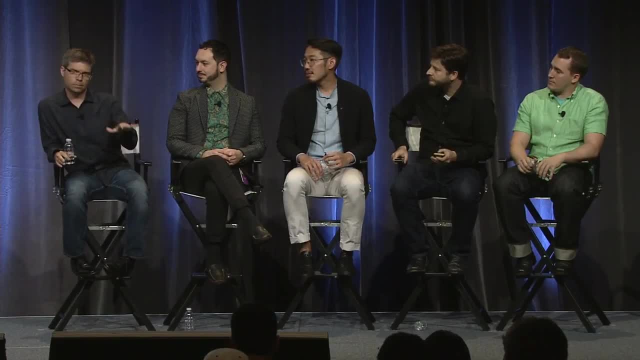 And so we just want to make sure that we're always grounding it into sort of these principles that we set up initially, so that it's always self-consistent, You don't get to a moment where you're like, oh, I did this thing and then it that didn't make sense. 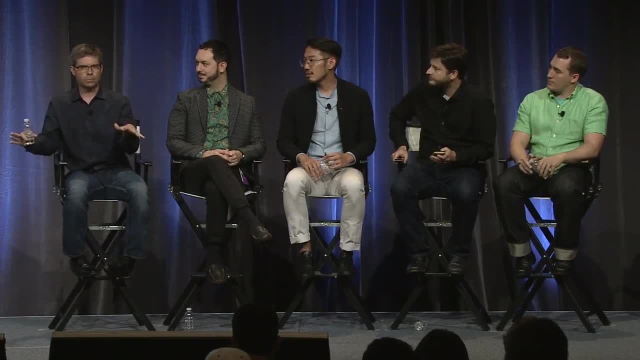 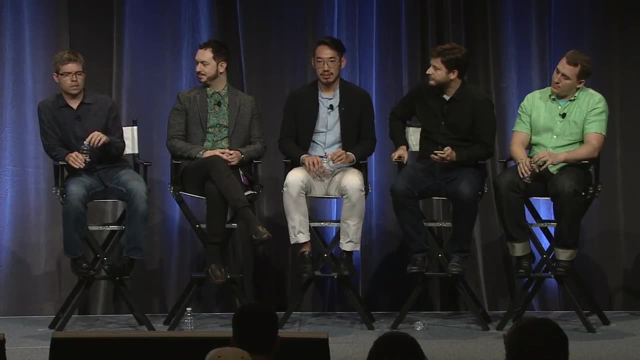 I did this, you know it was discontinuous with all of the principles that had been set up before it. One of the things that I think is really interesting about this- and we'll talk about this more in tomorrow's sessions- is that 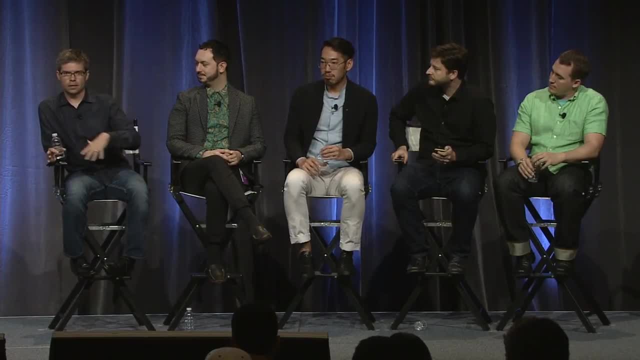 you know, there's actually a fair amount of spectrum right. There's a lot of different types of things that can be expressed both in terms of color and content, and the animation that gives you a pretty big palette right, It still feels like it's part of a system. 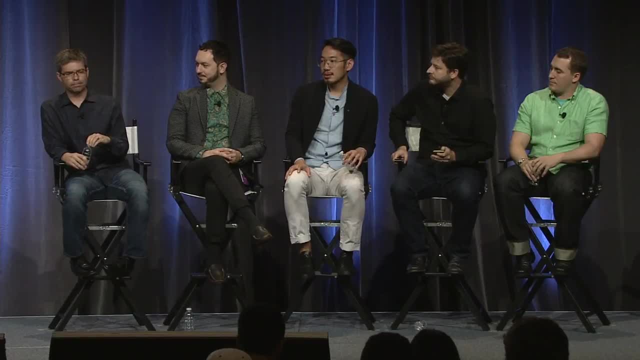 but it gives you a very large palette so you can express lots of different things. So, I think, the addition of wearables, I look forward to seeing how people express their apps and their applications through these additional different forms, different interface forms- OK. 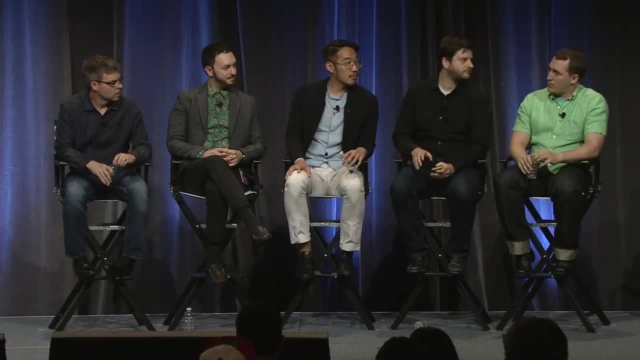 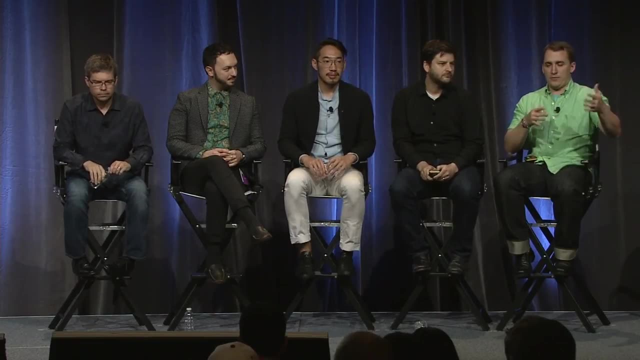 In terms of manipulation. One of the other things that came up as we were doing this first, as we were looking at just desktop and mobile together, was unifying the overall touch feedback through them, So having hover states and tap states all be resolved together. 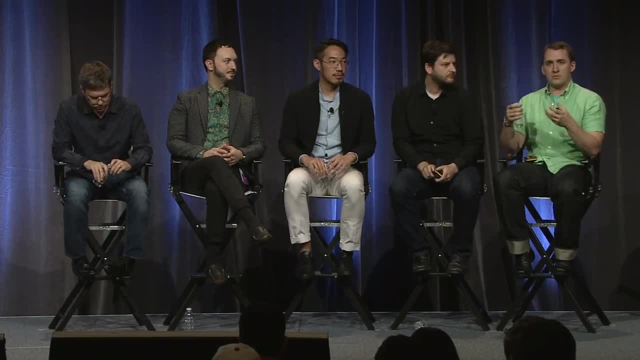 And then we started to see more and more of these And treating it as energy was a very nice metaphor for us, because we were able to look at on touch. these things are going to move outwards Voice. as you're speaking, you have a similar response to it. 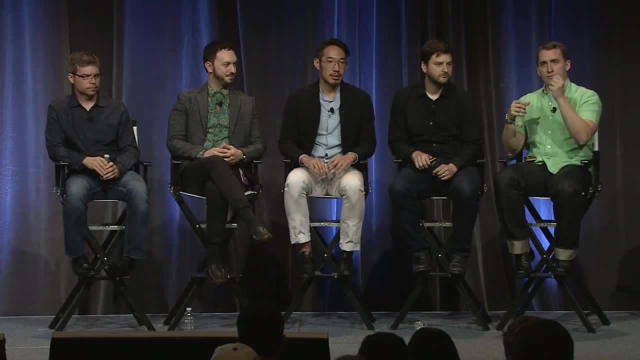 As you use the D-pad on the TV, the movement of your focus through a UI will be very similar And one of the things we didn't really touch on- but, like, tapping between controls using a keyboard can have a very similar feel of it. 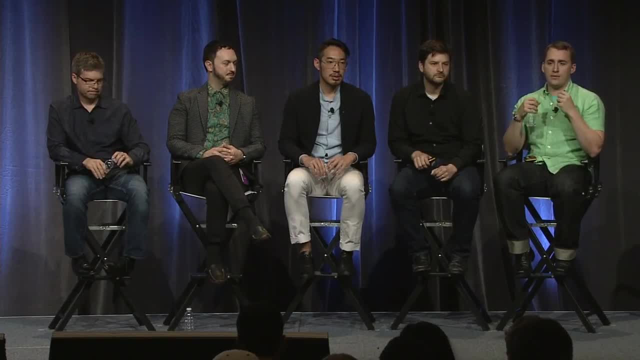 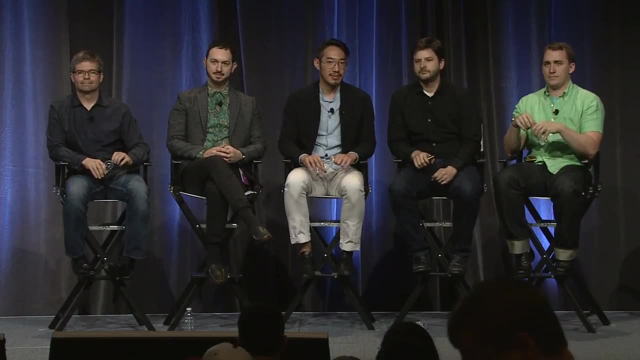 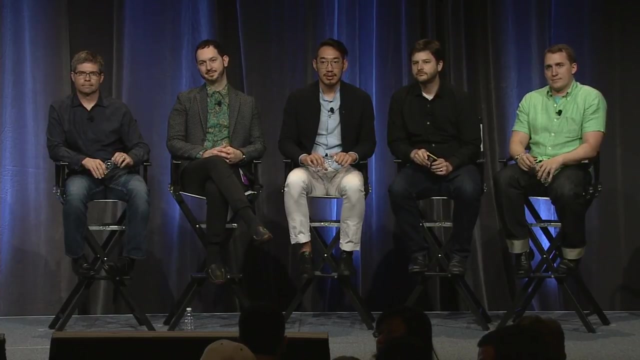 It is your focus moving through space And then, when you hit Enter on something that energy blast is very similar to any other mode of input you might do. Thanks, Thank you guys, Appreciate your time. So I work for a company where we are both cross platform. 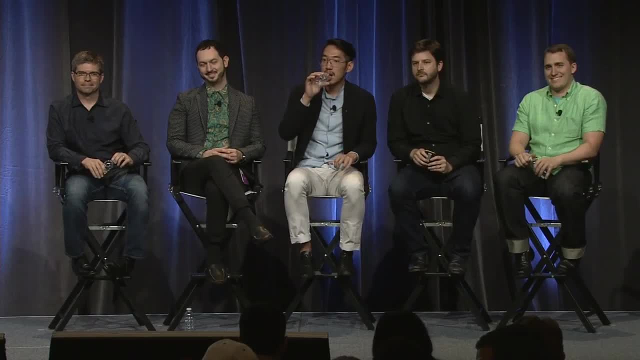 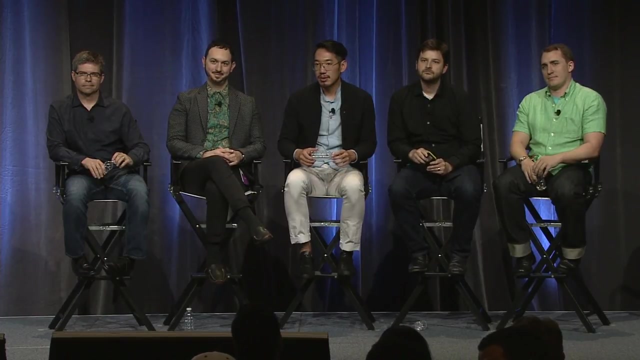 and our mobile apps are not our primary moneymaker. So, when it comes to time, So when it comes to requesting time be allocated to working on this, it can be looked at as a little bit of an indulgence. What would you suggest as some maybe priorities? 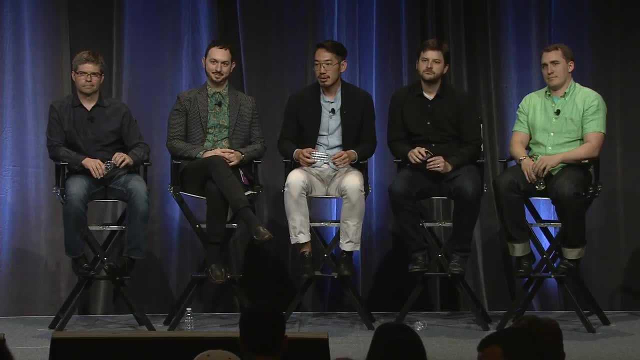 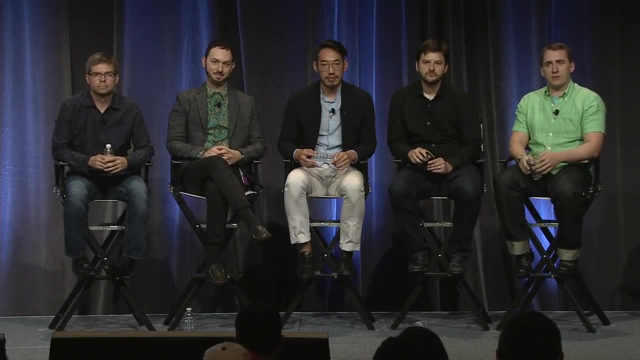 to focus on when looking at implementing some of these things. For the most part, the framework should be supplying 90% of the animation and the richness in the UI. What we're asking people to do is actually look at some of the new APIs for shared element transitions. 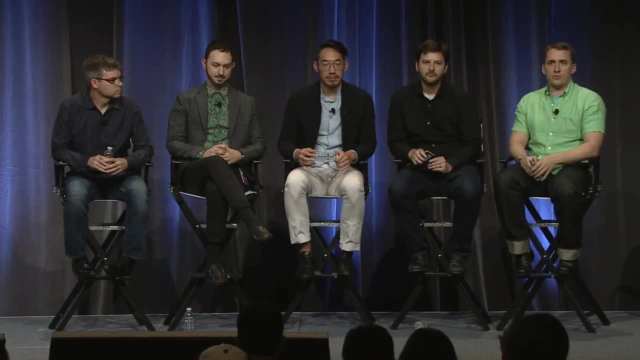 between activities. Like there are moments that may be a little bit of a challenge. but there are moments that may be a little bit of a challenge And so we're trying to make good places for polish and brand in your app. So, using the core elements, using the core iconography. 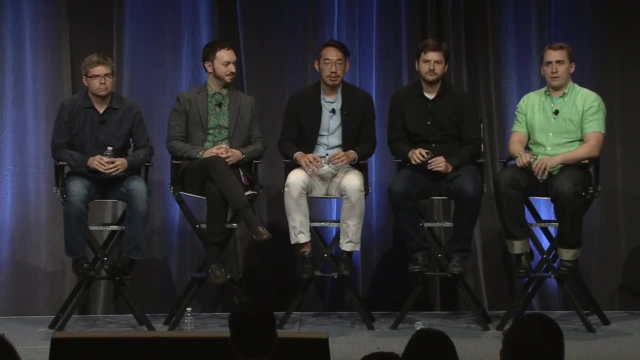 using the theming to make it feel like it's your product, but then just polishing one or two really critical things usually has the best outcome, And a Polymer framework is actually going to be really great for all kinds of different platforms- mobile platforms. Yeah, And part of the reason we've done this for ourselves. if we do a mobile web app and a native app, to create a very similar structure there so we don't have different interaction, designers thinking about different ways of handling it, They should be treated as pretty much the same app. 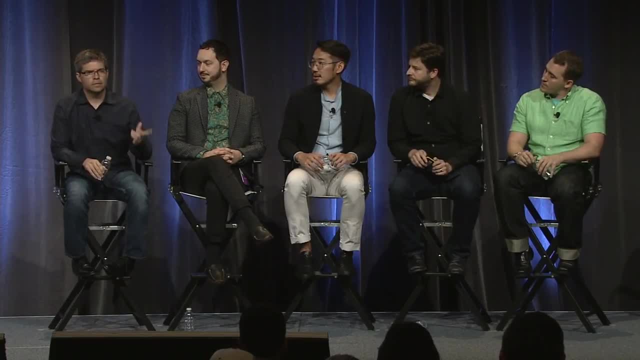 with small adjustments. It's probably a good opportunity to also mention that after this, we're actually going to go. some of us are going to be in the design sandbox on level 2. And, as part of releasing our spec and design and having all this announced, we really 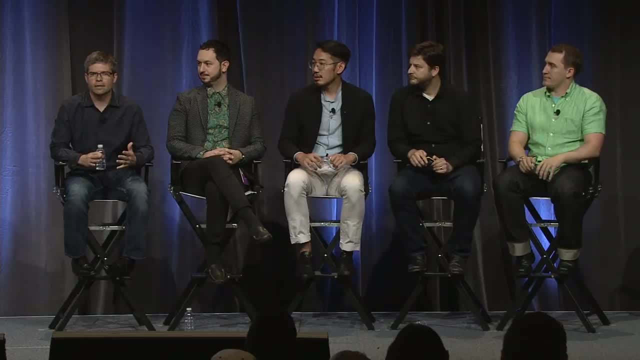 want to talk to designers and developers about kind of the problems they have in terms of what they're trying to solve for their users And so that we can understand how material design and the principles here can help support that. Or maybe there's some unique problems out there. 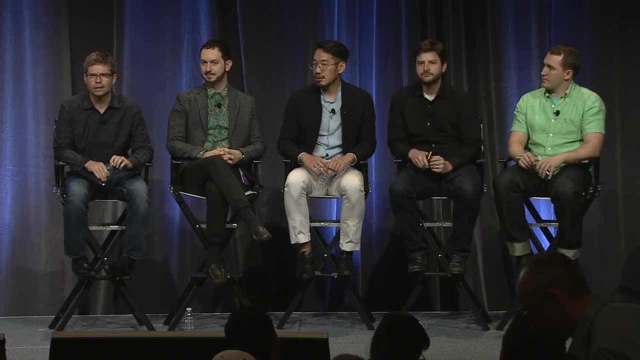 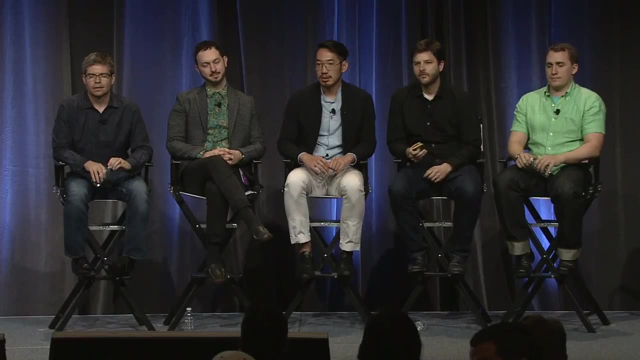 that need a little bit of a different twist, And we'd love to hear feedback about that. Cool Thanks, Hey there. I'm Peter. I'm a UX UI designer And my question is regarding animations For one. as you all know, animations 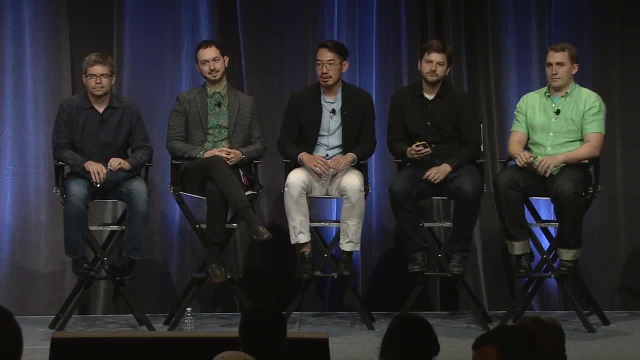 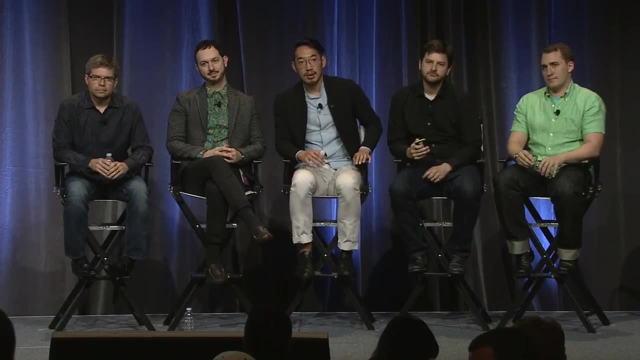 are something that kind of make an app pop and stand out, And recently we had a lot of trouble where I work in design agencies and stuff. So where we make an app, we create animations, either in After Effects, Origami, or we just animate them manually. 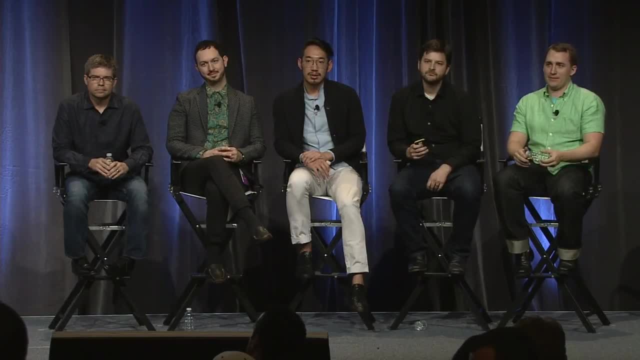 And I was wondering if there's going to be a tool from Google that will help us kind of animate our design, Because that's the hardest part of transferring it to a developer, explaining to them how it's going to interact, And will there be an addition to the design guidelines? 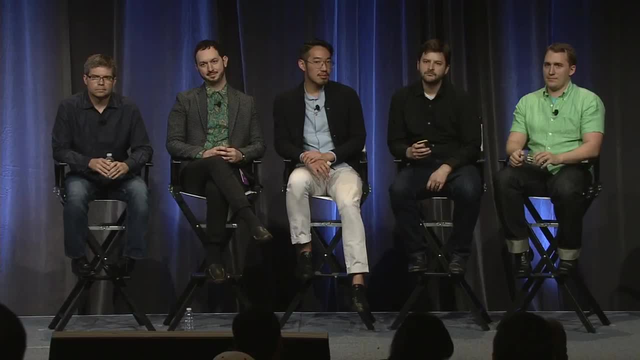 explaining what kind of default animations you should focus on. What kind of will there be like more of a sandbox that designers can use so they can kind of get and carry their points across to the developers? Because I usually find that point where you kind of transfer all of your work to the developers. 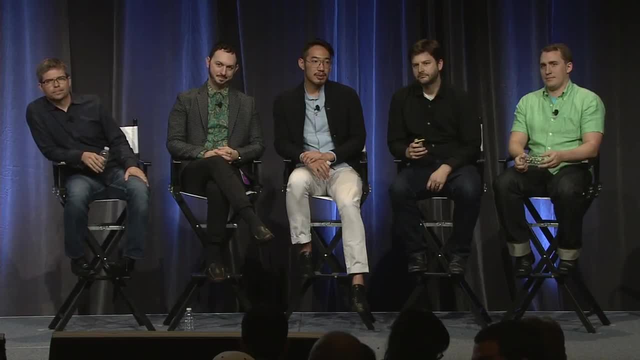 that's the toughest bit, And if a tool were there, like a native tool, that would help us aid in that process, that would be great. But do you have any tips for that And is anything planned on kind of like improving that? 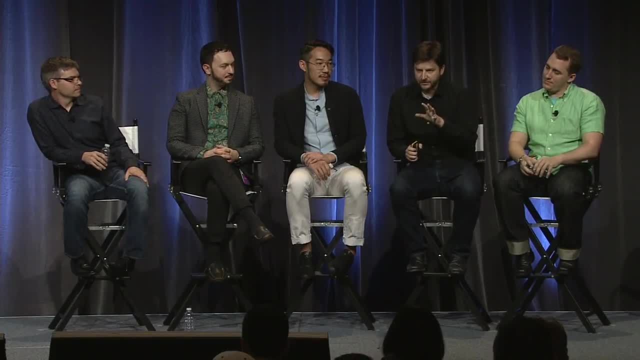 So, even before the tool, one of the things that we've noticed as we've been doing that same process and designing things and working with engineering to make them happen, is that having that shared metaphor and having engineering kind of understand those same principles gets us a lot closer from the very beginning. 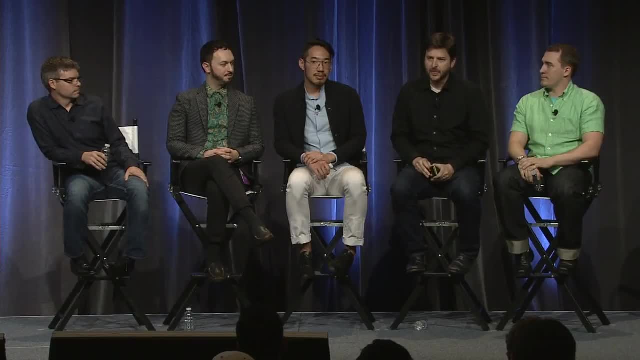 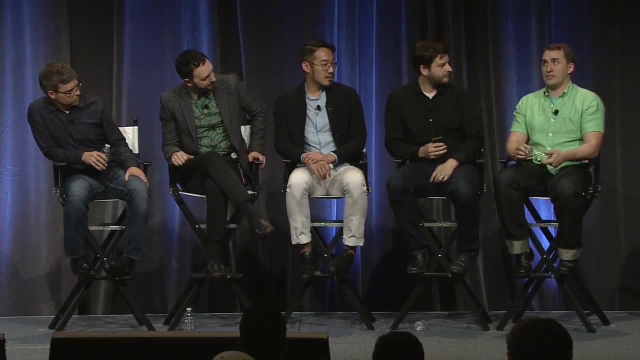 that we kind of know how things should move and how things should react, And I think that's a good place to start. I don't know if anybody else wants to comment. It's also helped us to. we actually define a number of different animation curves. 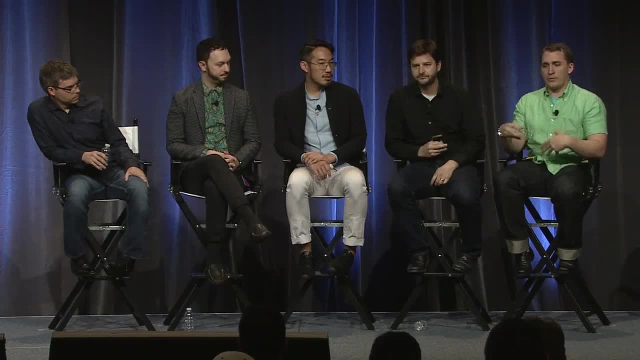 Like we're not using just sort of simple ease in, ease out, But we got those sort of built in and worked with the engineers so they understood those And we tend to use them everywhere and then we iterate on them as needed. So, tools aside, 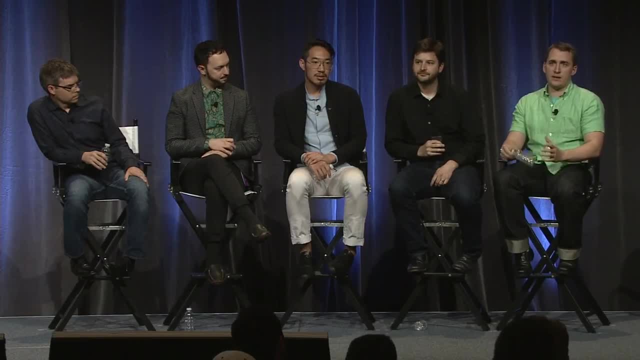 Yeah. So, tools aside, we found it just helpful to stay in constant communication with engineers and try to get as much of the stuff baked in as logic into the system rather than as things that we're handing over that are one offs. And what's your standard design process? 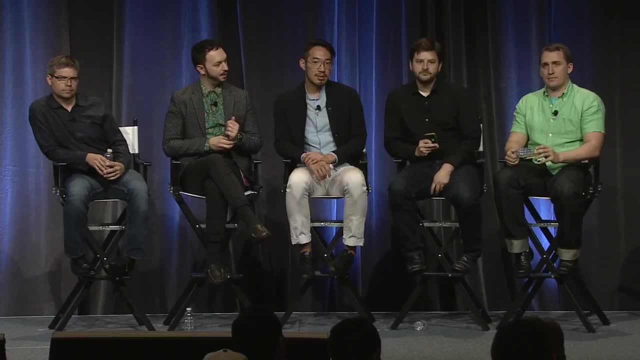 for explaining it to the developers. Is it just like a case of them sitting near you and you kind of covered the entire animation process with them together? How do you get the point across to them? It's fairly ad hoc, Depends on the situation. 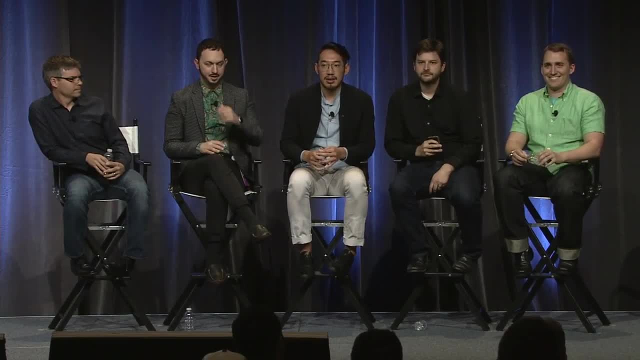 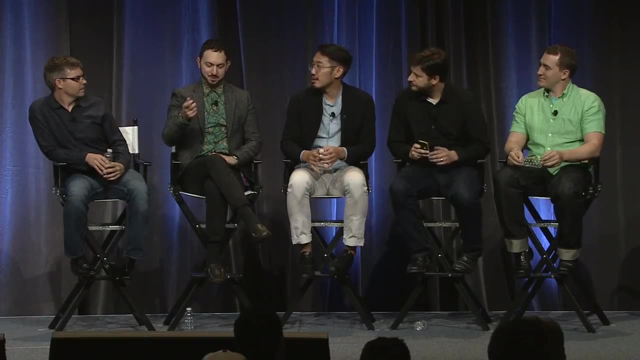 Sitting together is always the best way to accomplish anything. OK, I was just wondering if you have a standardized process for that. All right, cool, Thanks. Yeah, I do want to mention before you walk away that that kind of request or interest in tools 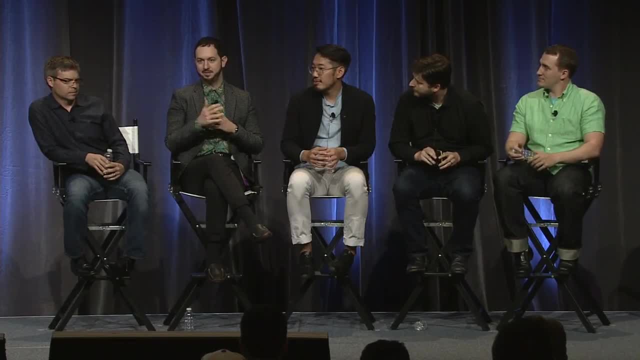 or anything like that. we don't have any tools to announce today, but that's the kind of feedback and pain point that you guys are feeling, that we'd love to hear about more so we know how to focus our energy, And if you guys have more of those kinds of questions. 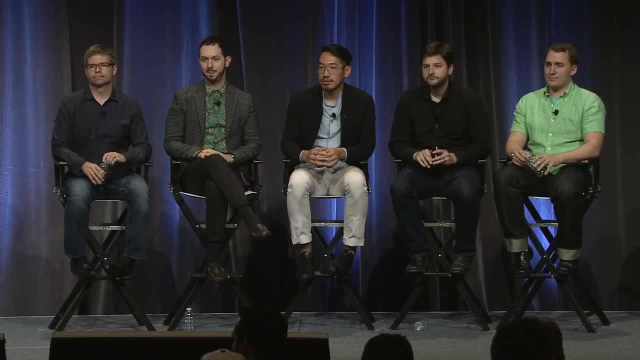 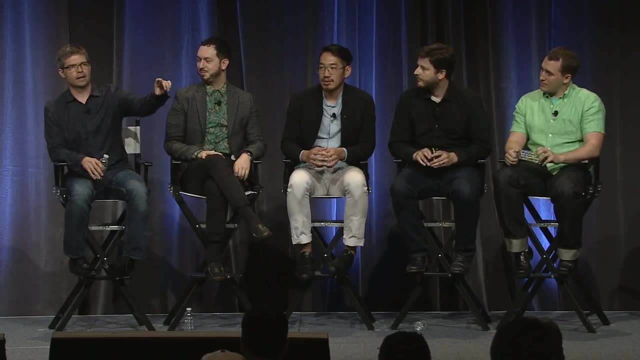 or requests come by the Design Center. Yeah, it's called the Design Sandbox. Wouldn't follow up. Where's the Design Box? Sorry, It's the second floor. It's design. It's over by the Distribute section, Kind of like you look for the YouTube sign. 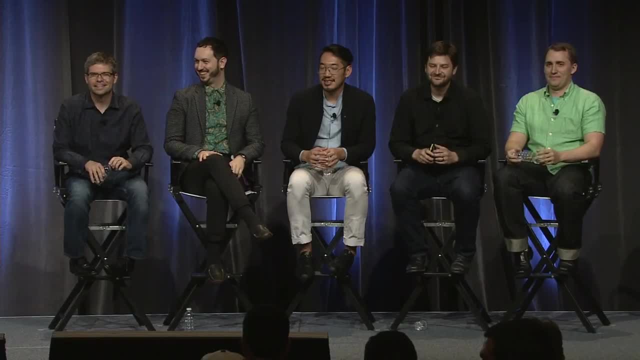 Oh, so it's downstairs. Yeah, it's by the YouTube booth. It's a very clear design, Yeah, So my question is really about color, And I see a lot of bright colors these days everywhere And even in the pictures there. some of you 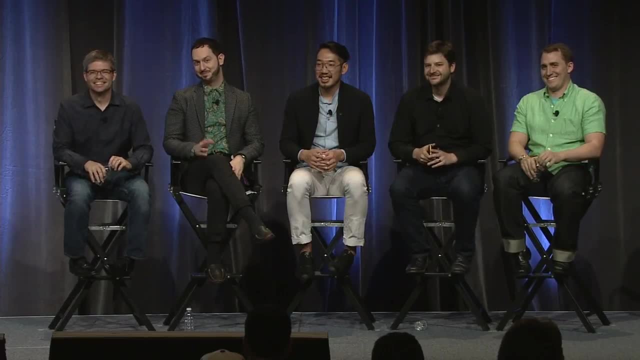 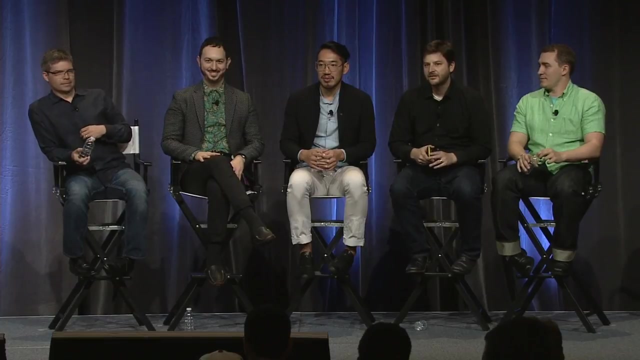 have a purple background and a red, So very bright colors, and they're all different combinations. So how do you pick these bright color combinations in context of material design so that it's actually appealing to the user and it has meaning and it's not bright enough to be noisy or something? 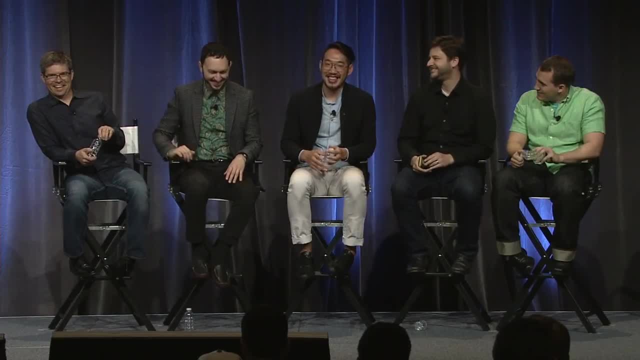 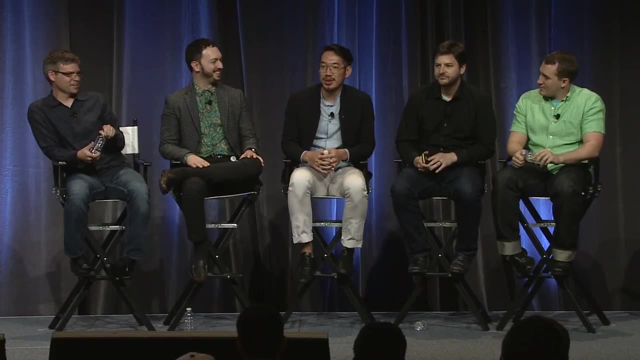 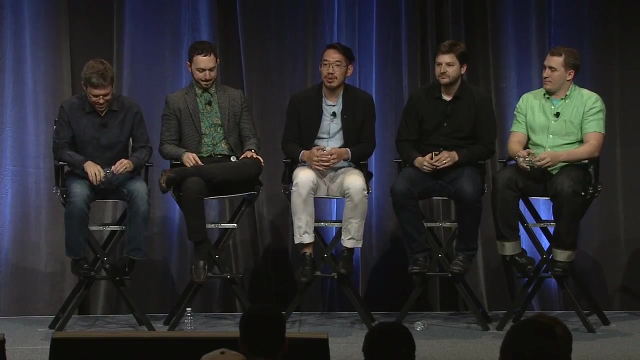 We test 41 shades. Not funny, I think it actually is Just kidding. Just kidding, Sorry, Too soon. There's two approaches to color. One is that we intentionally wanted to take a very exuberant approach to applying color to our applications. 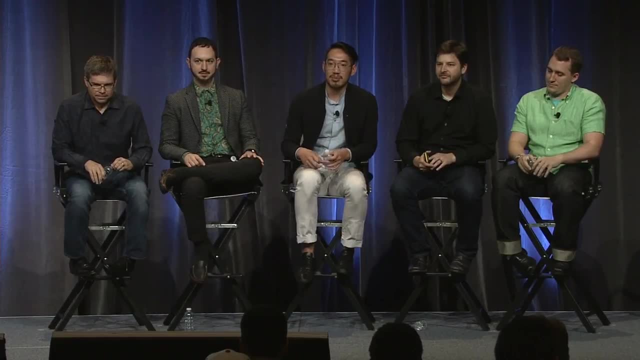 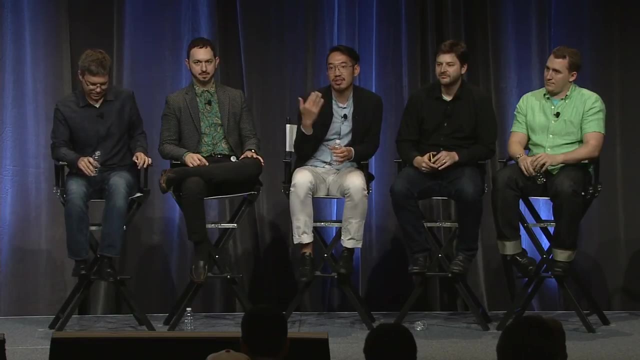 We felt that, like I was kind of talking about some of the slides where you should really embrace your brand's product colors or your icon colors and extend those things all the way through All the series of screens that someone's going to see- 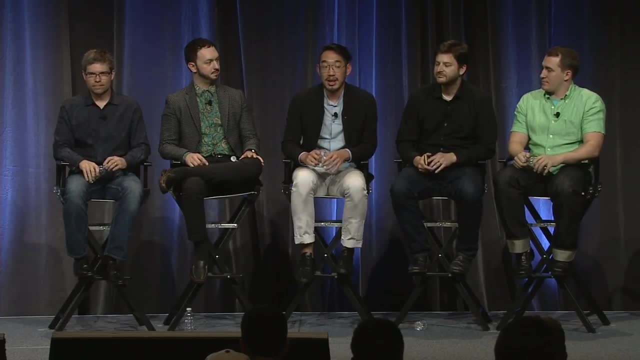 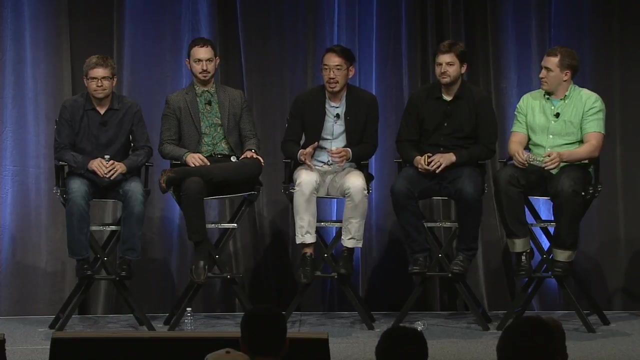 And so we thought why not push it further? On the reverse side, I think there's also some pretty extensive usability and contrast ratio studies that we've started to standardize around, And I think that that's the intention of the design guidelines- is to kind of help give guidance. 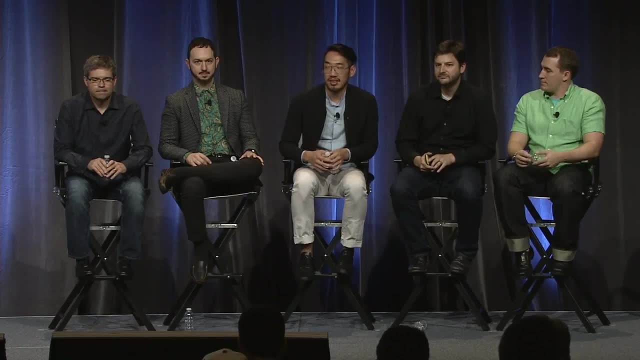 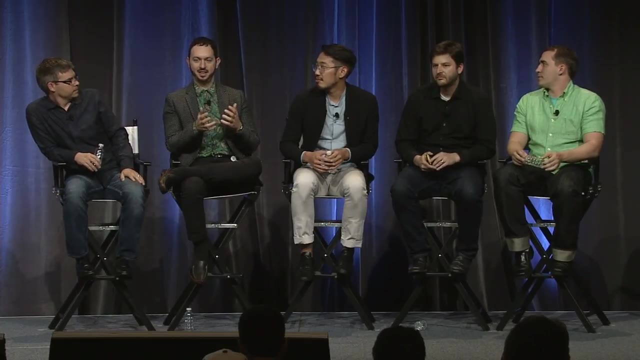 on being exuberant while still being accessible and usable. Yeah, It's super clear. if you go into the spec, you will find a whole bunch of palettes And they have a lot of guidance on what kinds of colors you should put together in order to get legible text on top. 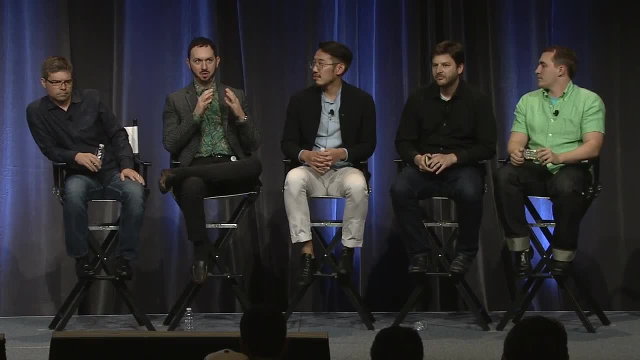 of them and stuff like that. But we are very much in love with and excited with these modern, bold colors. But the entire system is designed to let different approaches and philosophies to color feel just as much at home if you want your content to pop. 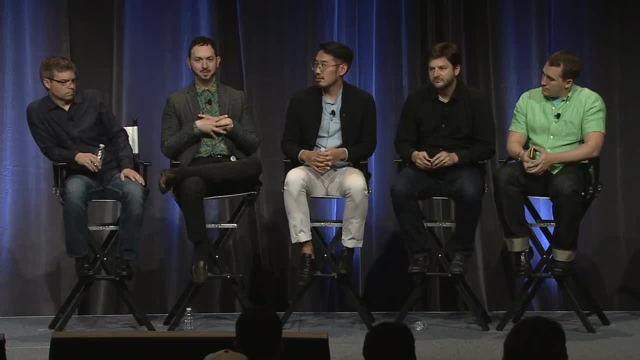 more and your UI elements to be really muted and subdued. That's part of material design as well. The idea is that it is a material like paper And you can print something that's very exuberant on it, Or you can print something that's much more muted. 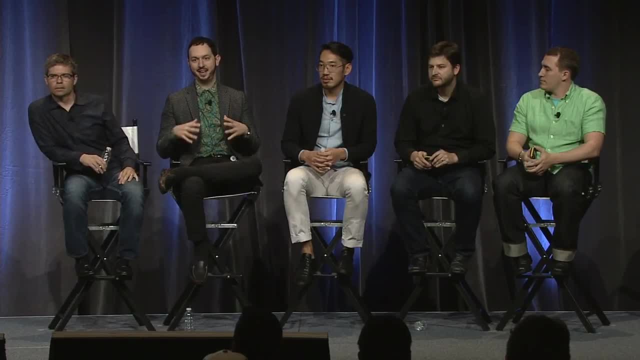 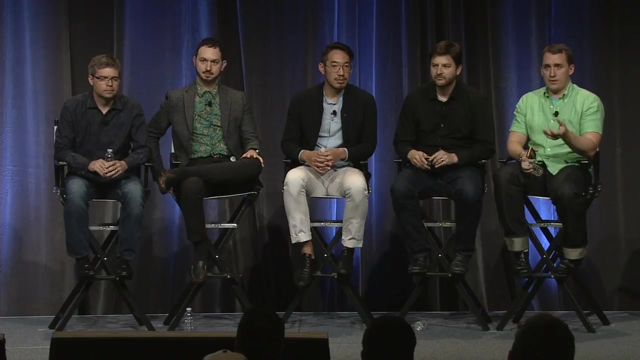 We want it to be a framework where any brand can fully express itself and feel at home and not be overshadowed by the platform's conventions. Some examples you actually can look at in the preview will be: the Settings app is quite muted. It's intended to be very utilitarian. 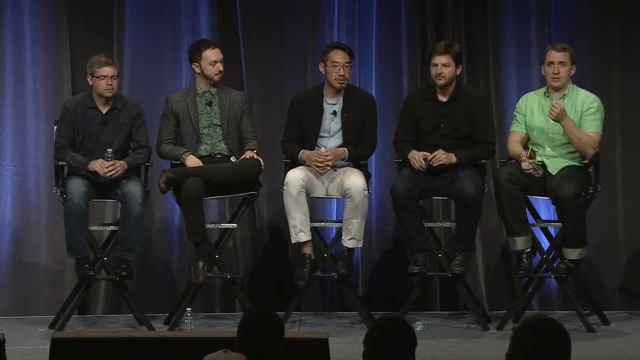 Calculator app is also muted, but it uses a single pop of color to draw attention to other functionality. So it's again about management of where you want attention and color. that makes an app really unique. One other point, too: the palette library. 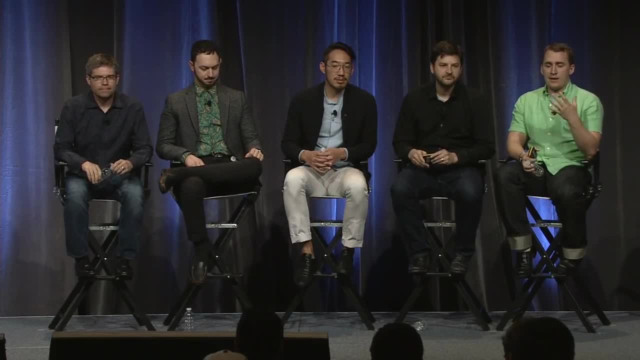 that we've been working on. One of the reasons we were so excited about it was it allows you to select colors that can go alongside imagery, that allow the image to feel like it is covering the entire surface, rather than an arbitrarily chosen color that may contrast. 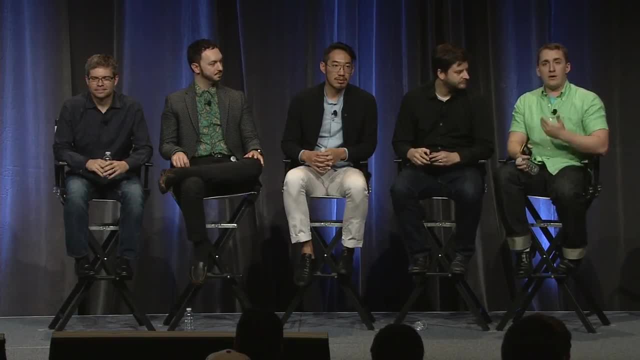 in some unusual way. So you have the opportunity to have it extend the image outwards into the system, or even to contrast with that image if you want to draw attention to an action. It looks like we only have three minutes and four questions left, so let's try to get through them super quick. 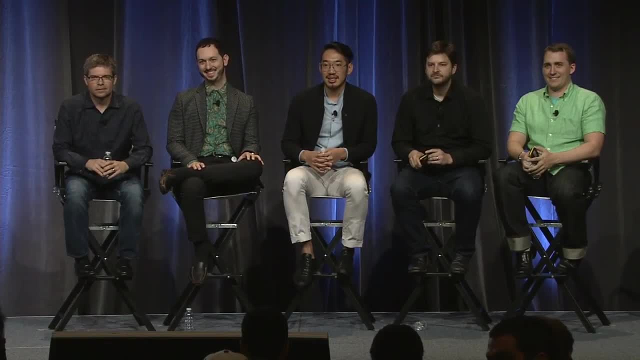 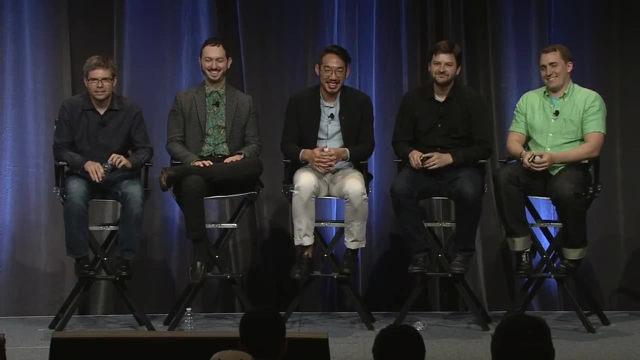 I'm sorry to take the time, but actually I have two questions and it's tough. All right, thanks, The crowd will vote on which one we answer. No, just joking, Go ahead. First of all, I heard Jonathan is working for UXA, which 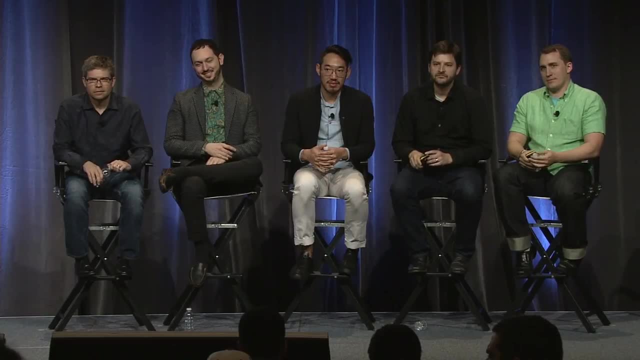 is the Google Define Cloud And he's working on the UI guidelines for the Google Apps, So would you like to talk about that a little bit? How would you work across different apps to make the UI's guideline consistent across Google Apps and how you also make sure all the apps will follow? 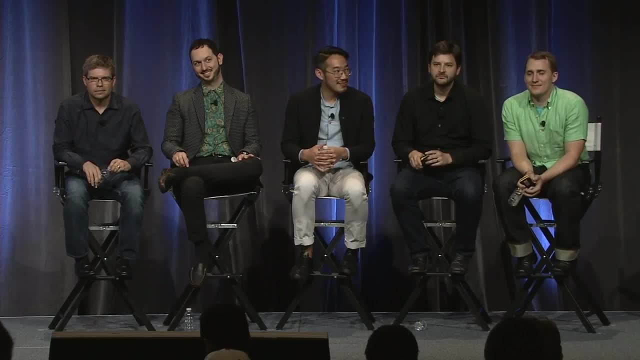 the guidelines when you did that? That's the first question, And the second question was Google always have a big push on the left navigations? As a company, we did follow that rule And unfortunately, what happened was after our release from main screen navigation. 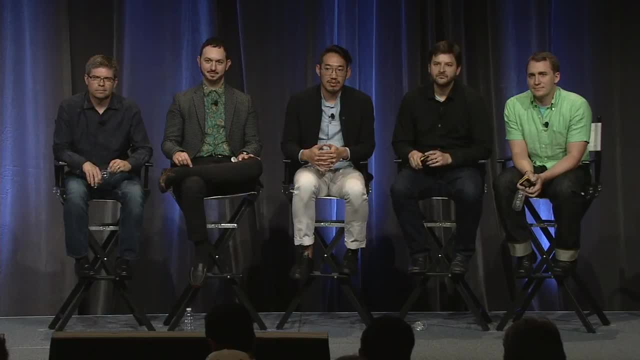 to the left navigation. we did see a lot of drop for user engagement And also we see a big trend that for Facebook app and Google+ they changed from left navigation into the main screen navigation. So do you guys like to share some insights of that change? 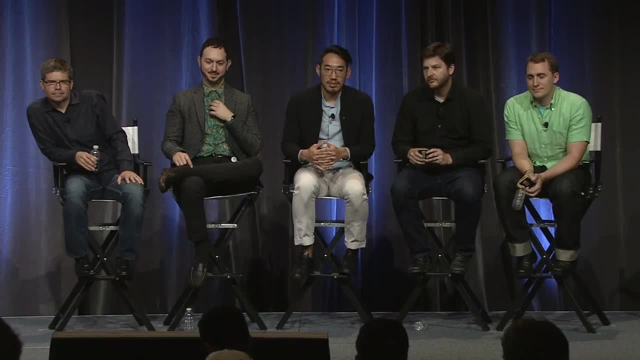 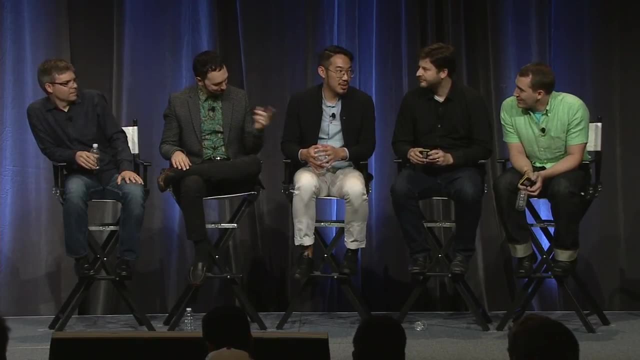 and how that will lead into a lot of companies that develop social apps that could get insights from this. Thank you, OK, I'll answer the second question first. Super quick second question: Left Nav is appropriate for certain classes of apps- The places we've seen the most successful. 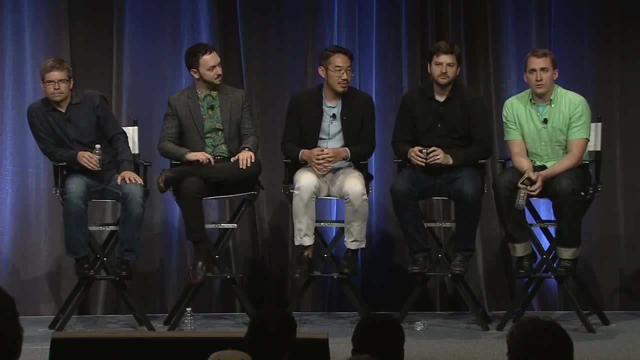 is when it's something like Gmail or a stream of content where 90% of your time is spent there And the rest of the time you need sometimes access to other labels or things like that. We'll go a lot more into this in interaction design. 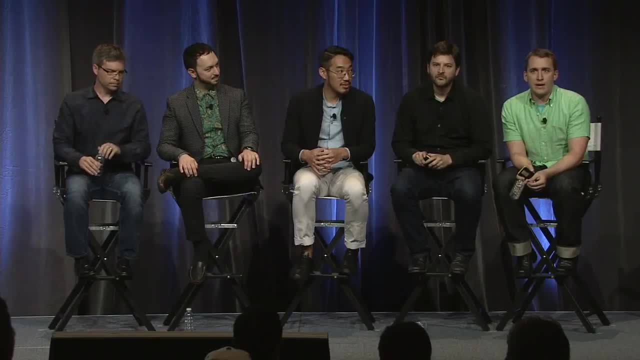 tomorrow morning. but Left Nav is only one of a number of different top level constructions. You can have tabs, You can have the content area itself act as overall navigation. One of the things we are trying to do in the guidelines is very specifically calling out the benefits. 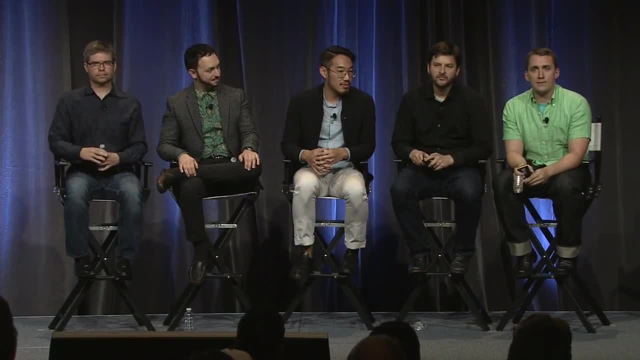 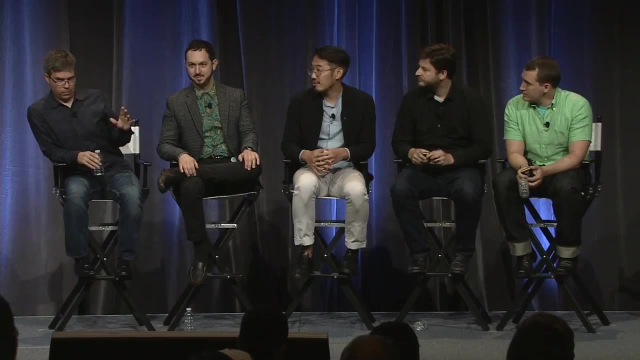 of each of those different ones. Left Nav itself is inherently bad, but when it's used for the wrong type of application, it can focus the user in the wrong way. And I'll answer the question: how do we coordinate design across Google? 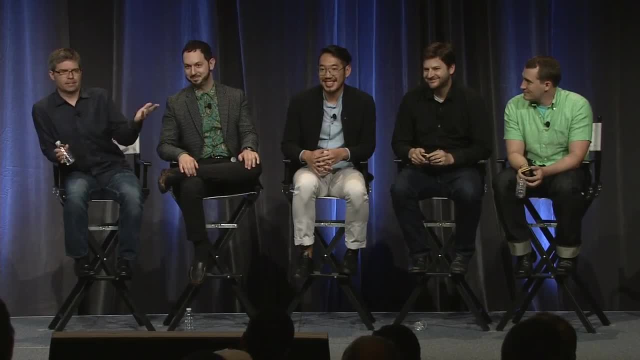 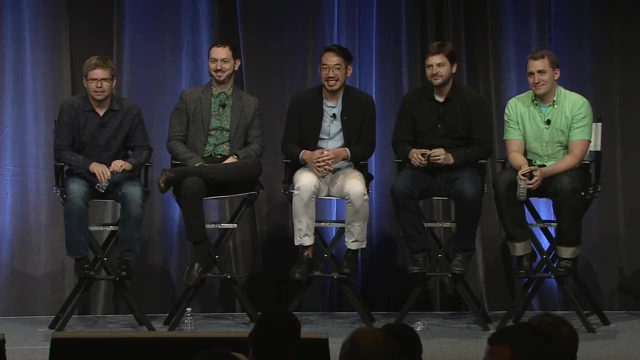 We all talk to each other all the time. That's it. We go out. we just talk to each other all the time, Just talking. All right, next question: Drinking and talking. I was thinking about all the material and the physicality that you stressed out. 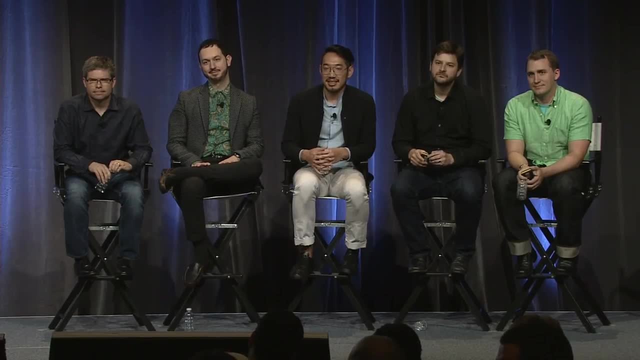 in the paper metaphor- And I was thinking about Facebook's paper app- And they go a step further, giving away all buttons and making the motion the clue to the interaction, like to close something And I wanted to know what you think of this. 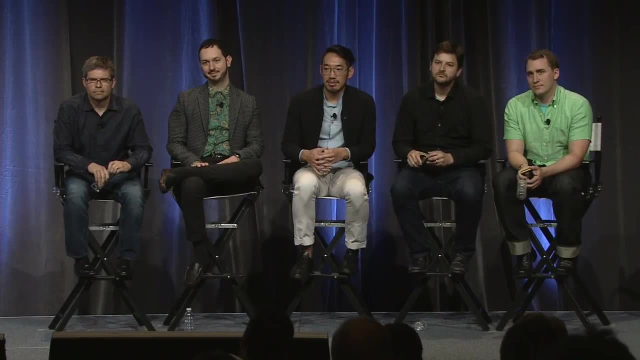 If you think that this app would feel right in the next generation of Android apps. We love using motion as an affordance for things that can happen. We need to be careful about being too reliant on it, because there may be people who can't perceive it. 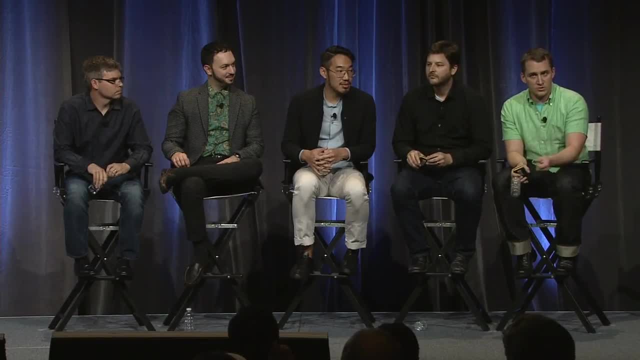 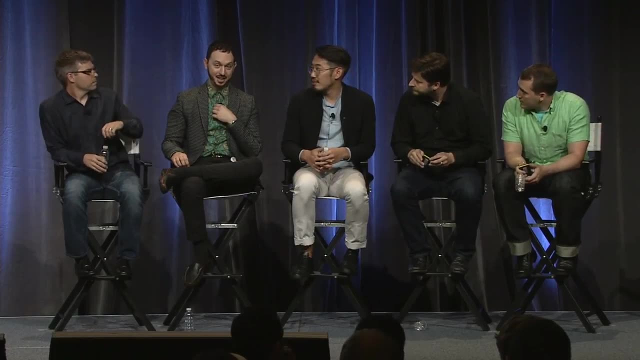 But it is a wonderful way to give clues as to gestures that can be taken and even just to simplify the way the UI looks through it. So we're excited about the possibility You can see in our calculator app we have a side panel of expanded options. 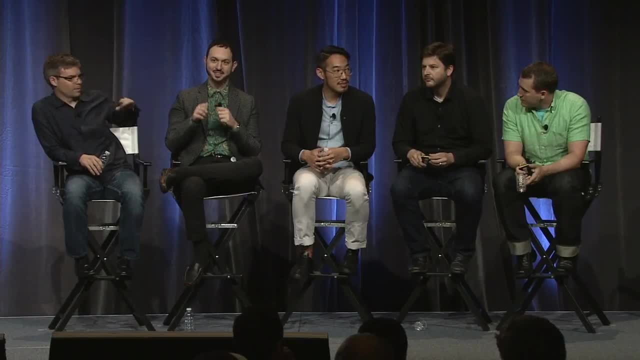 There's no button for it, There's no little textured drag handle, It's just a surface And you close it by a button. OK, And you close it by sliding to it? Yes, All right, We take one more question. 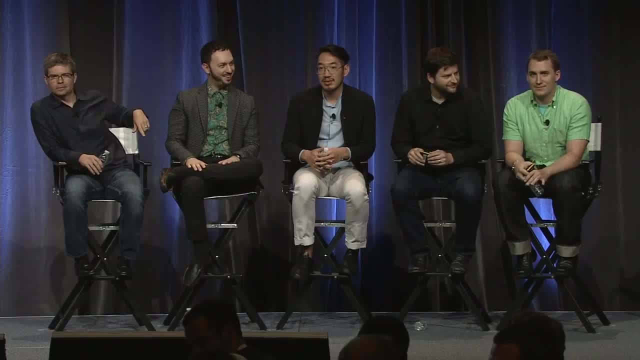 Oh no, Come on, Just one. Sorry, They're telling us to go. Hi, I was wondering if these design principles also apply to Google Glass. Google Glass: Will the design principles also apply to Google Glass As of right now? our design principles: